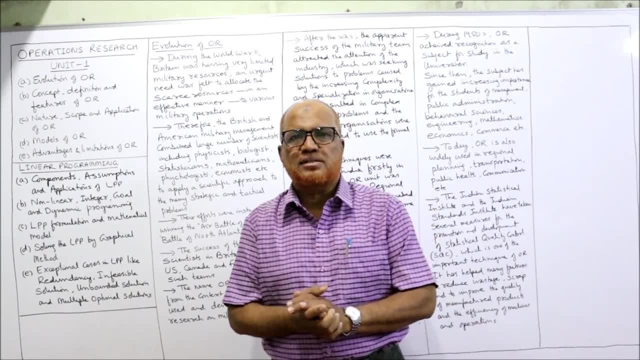 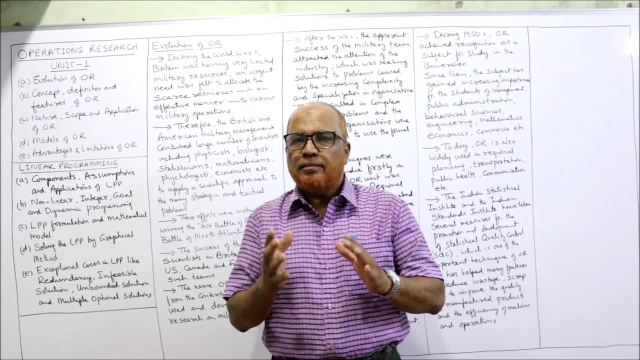 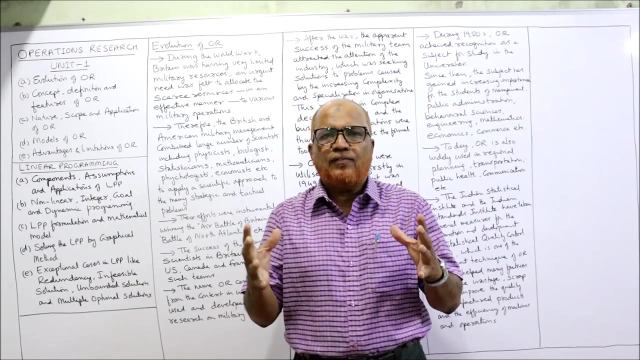 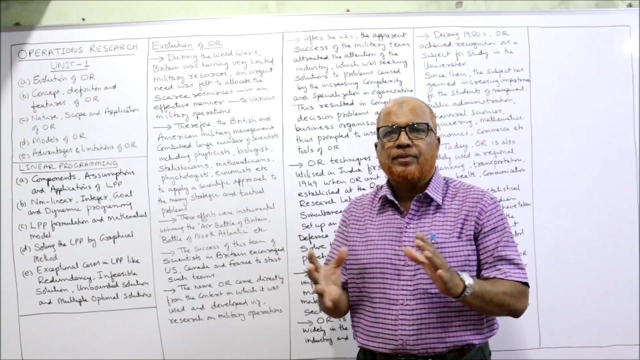 This subject is little bit tough compared to other subjects like accounting or statistics. So now I have decided to start the subject of operation research. This operation research subject is very important for management students, even for engineering students, For different categories this subject is there, That is operations research. Now, totally five units I'm going to cover in this subject of operation research. The first unit: 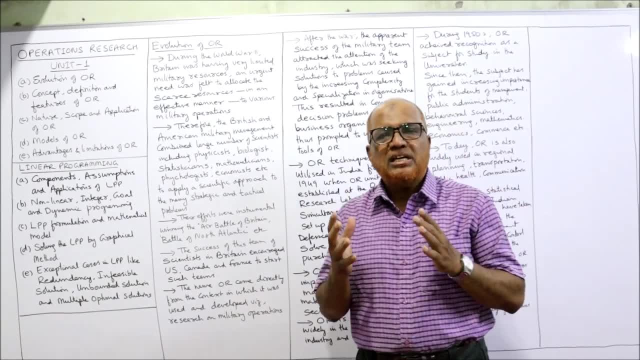 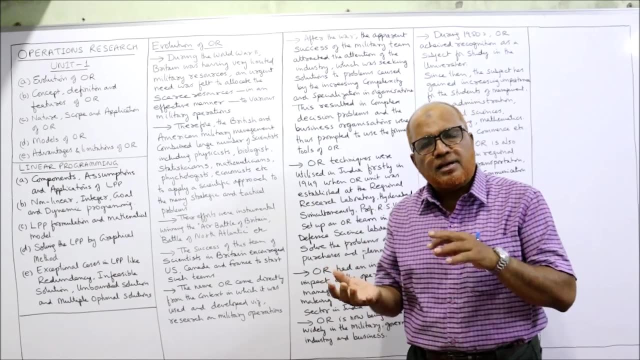 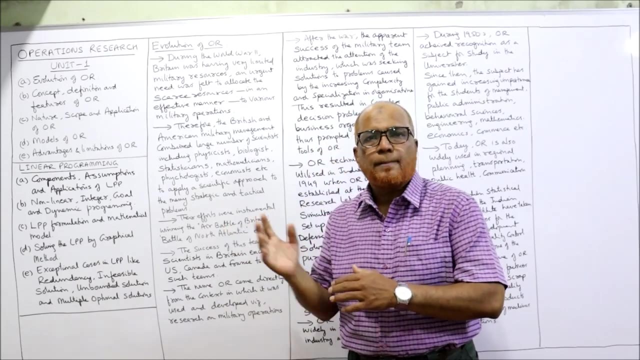 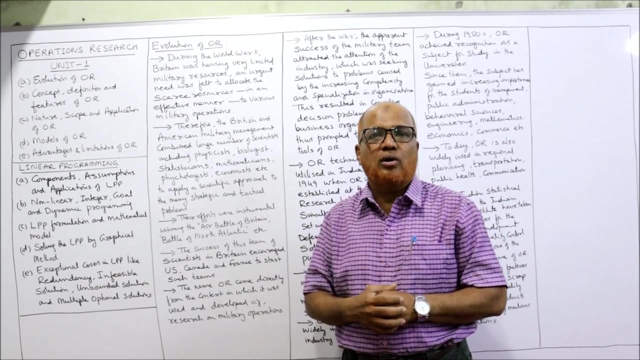 is the subject, the meaning, evolution, When it was evolved, this subject, operation research. Actually, operation research is not an old subject, Just like engineering, medicine, law, accounting. These are the old subjects coming from centuries. But this operation research has recent origin, So when it was evolved, how it was evolved. In examination you may get a question like explain the evolution of this operation research? 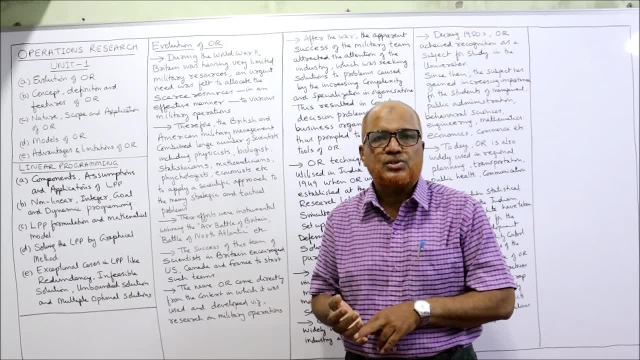 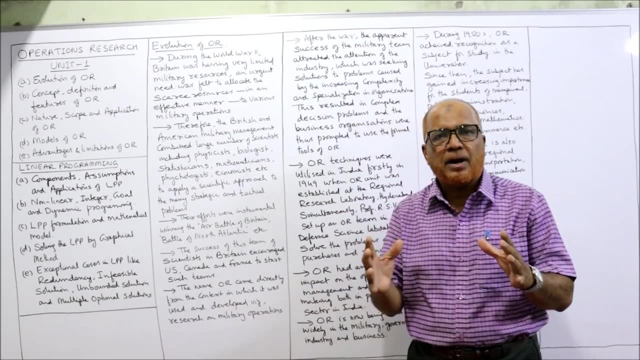 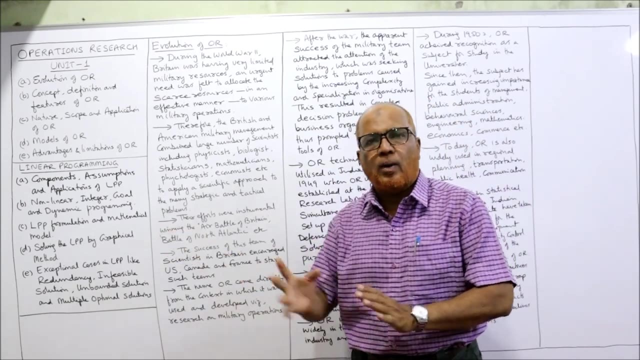 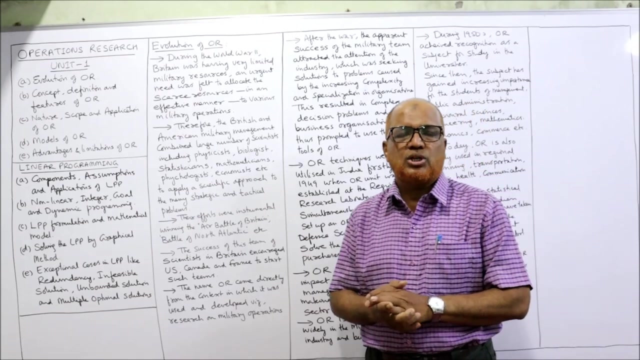 What is the meaning, definition, features, application, areas of OR, advantages and limitations of OR. So first part, I'm going to explain you about the subject OR, Then second part of this unit number one consists of linear programming. Linear programming is a technique of operation research in solving a complex problem where we have limited resources. 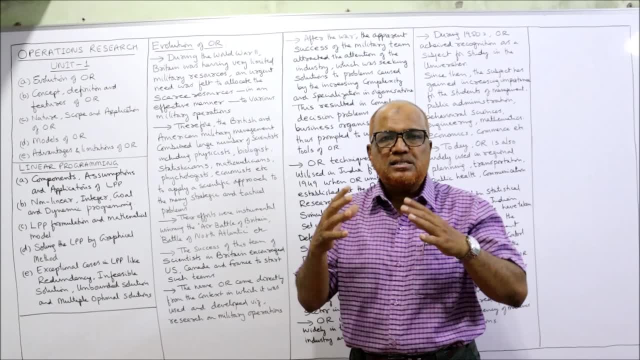 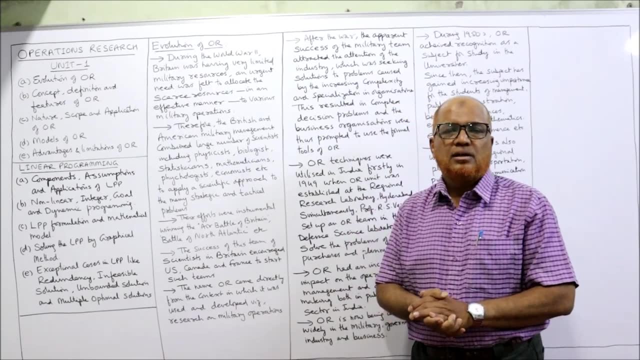 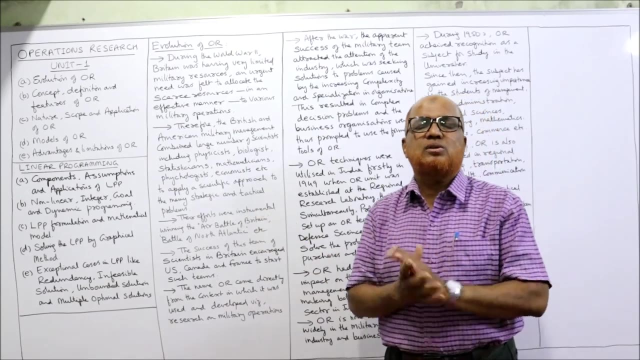 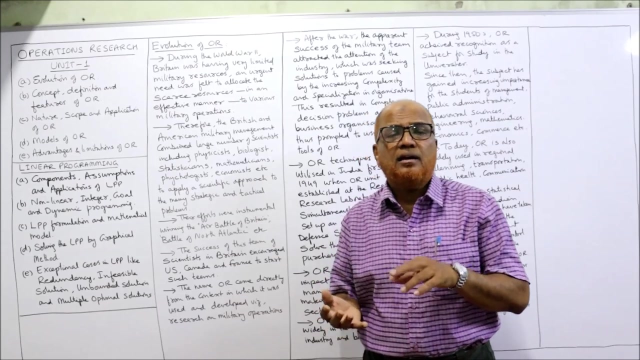 So how to attain the objective of maximizing some factor or minimizing some factor when the resources are scarce? In that case we apply the technique called linear programming. So what is the meaning of the term linear programming? What are the assumptions of linear programming? Application areas of linear programming, Different programming, problems like integer programming, non-linear programming, dynamic programming, goal programming. 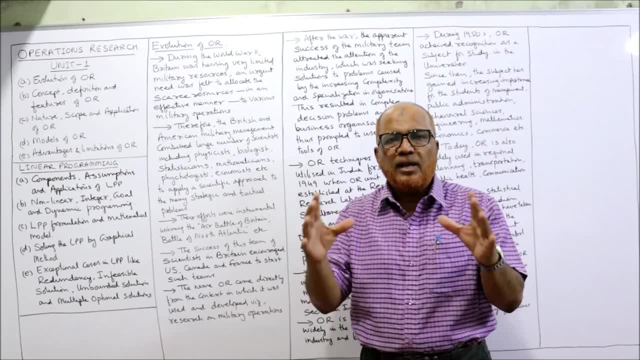 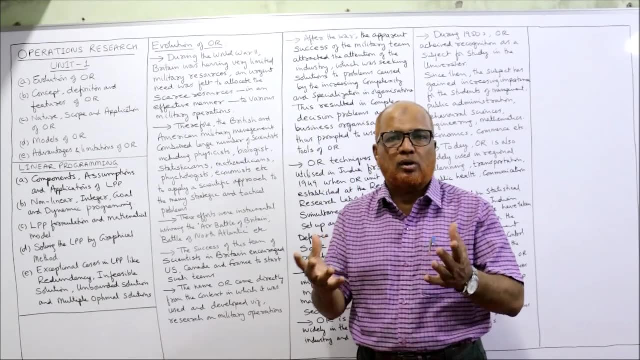 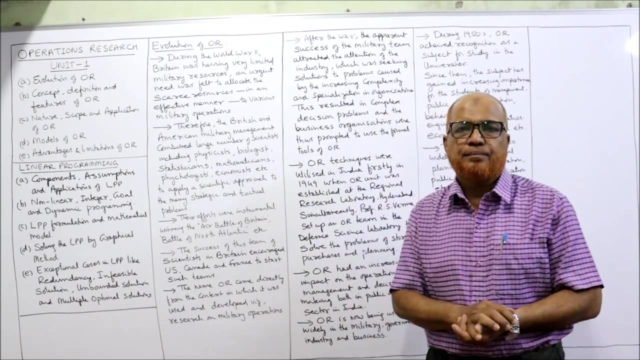 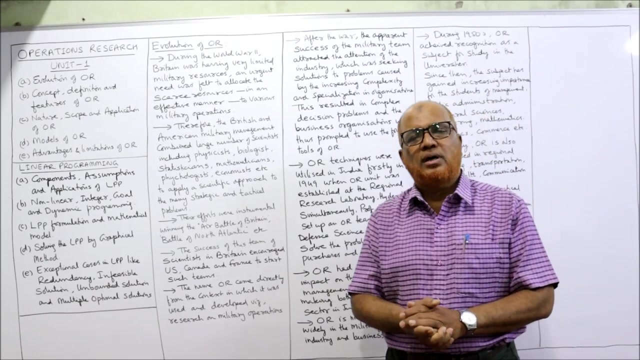 Different types of programming are there Then formulation of LPP, Linear programming model, Mathematical model we have to set up before solving the problem. Then we have how to solve a linear programming problem by graphical method, How to find out the solution of linear programming problem by graphical method. These are the things I'm going to explain in unit number one. 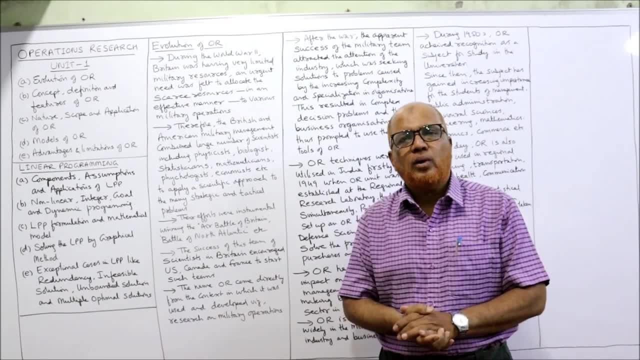 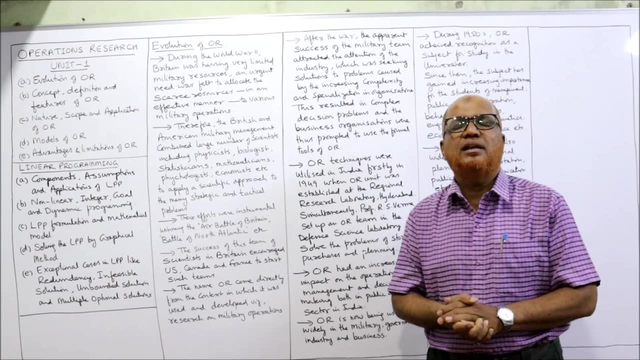 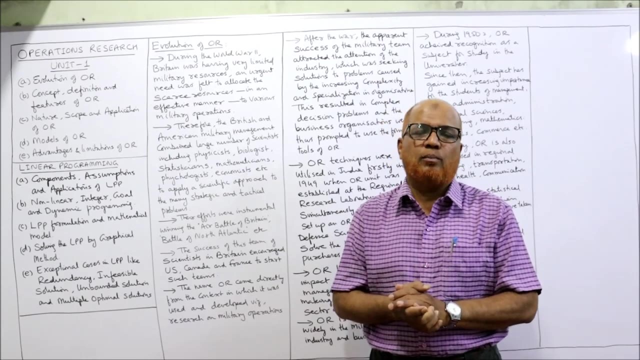 Then unit number two, Then system of allocation model. In this I'm going to explain you about the simplex method of solving the linear programming problem. Maximization problems, minimization problems, then duality problems, All these things in unit number two. 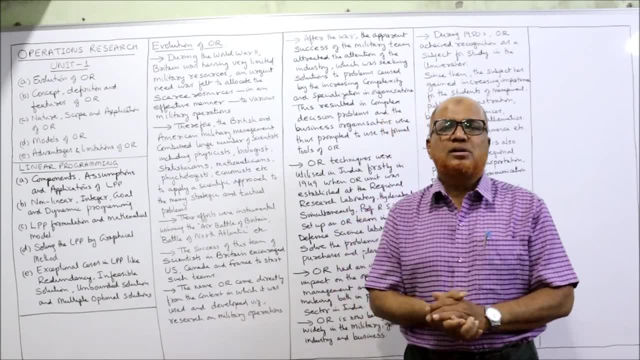 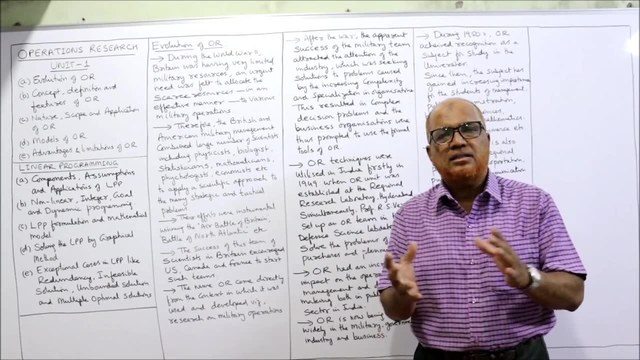 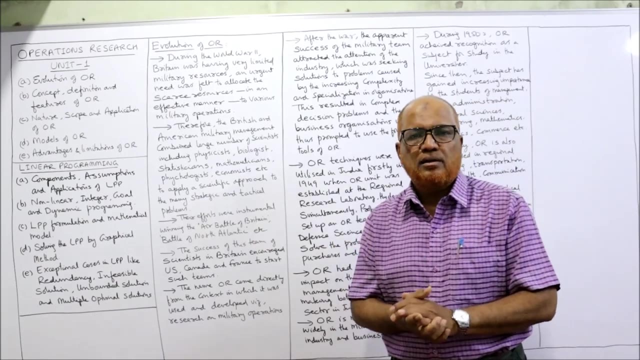 Unit number three: again, allocation problems, Transportation problem, traveling salesman problem and assignment problem. These are the things which we will discuss in unit number two, In unit number three. Unit number four: Network analysis. What is a network? Graphical presentation of a complex project. 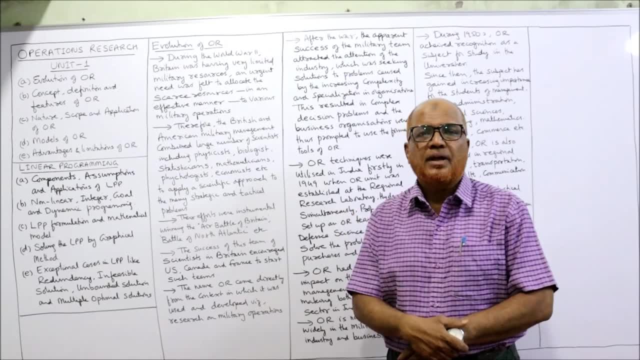 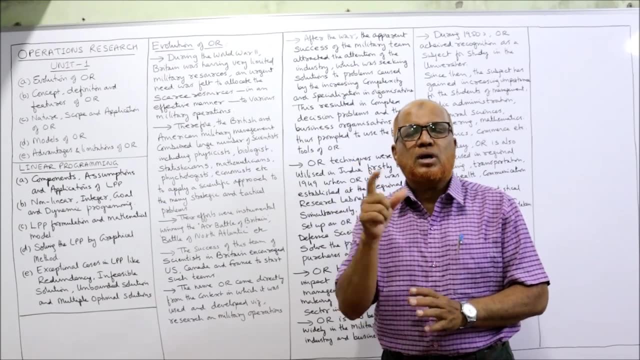 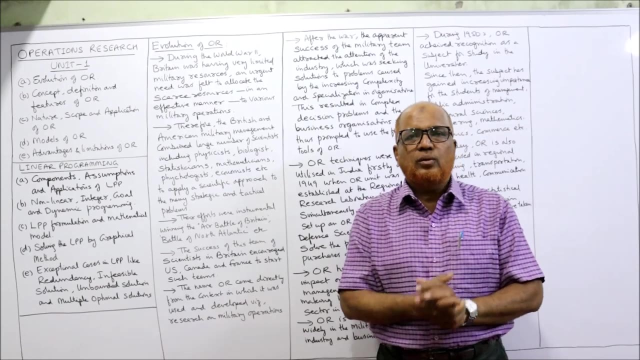 How to finish the project within the limited time and within limited resources, Then how to crash the activities. What is the estimated time to complete a project, So that we are going to discuss in unit number four, Network analysis, Last unit. The last unit consists of: 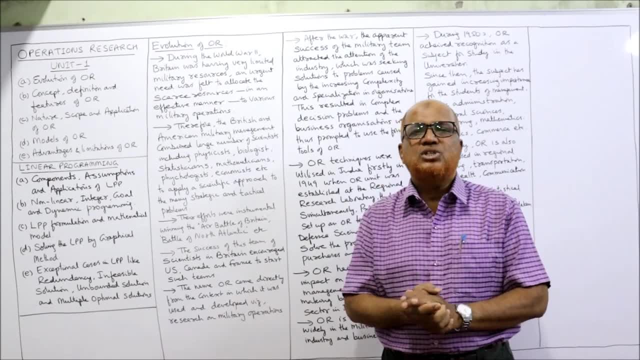 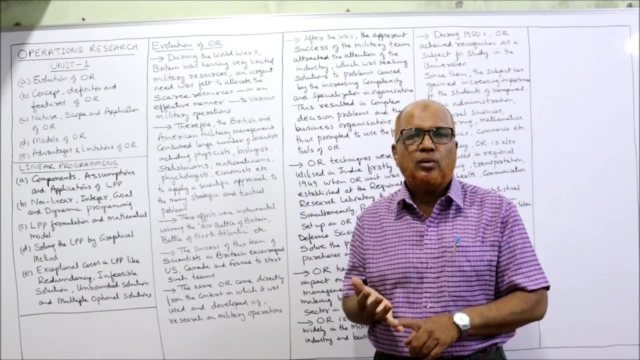 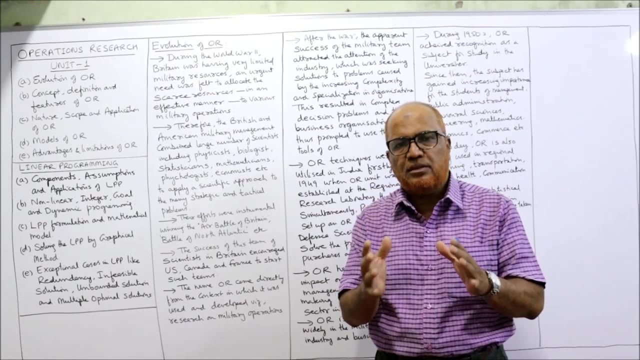 line problems, strategy problems or competitive situation problems. in this unit, number five, I am going to explain about the queuing theory, game theory and simulation. these are the complete topics of operation research I am going to cover up in this subject. so before that, in this video, I am going to explain you. 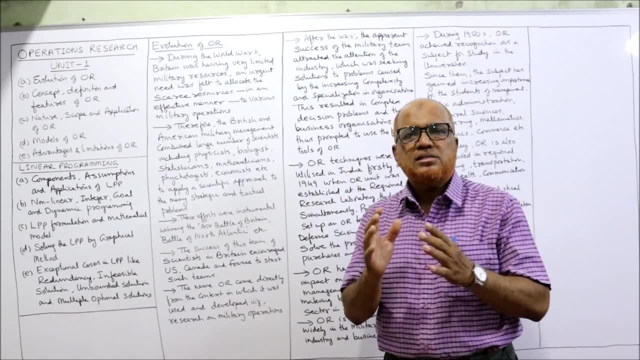 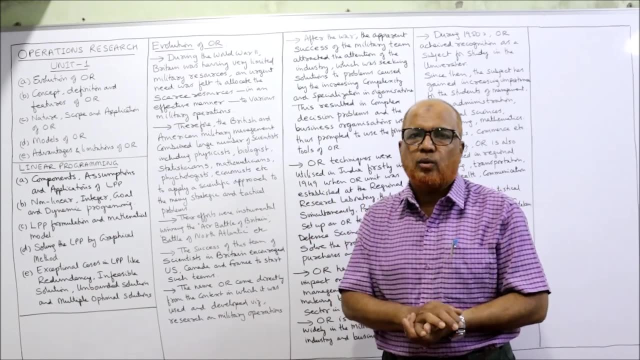 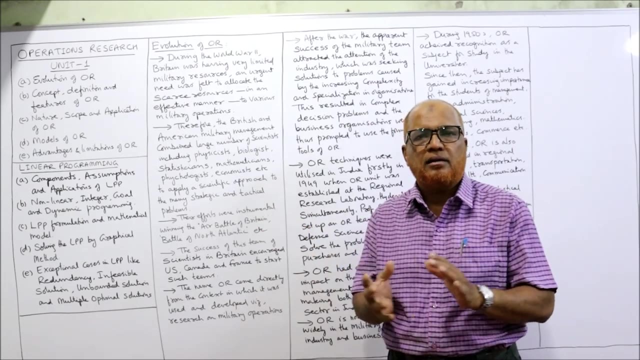 the first topic, that is, how this operational research subject was evolved when it was started. how it was started. that's what I am going to explain. so, before going ahead, take the screenshot of the points which I have written on the board. then I'll explain in detail. regarding the subject: operation research, 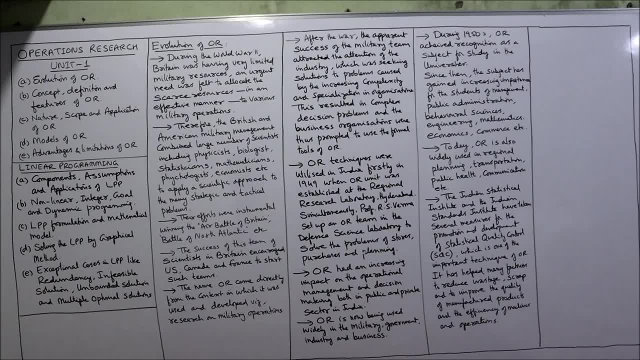 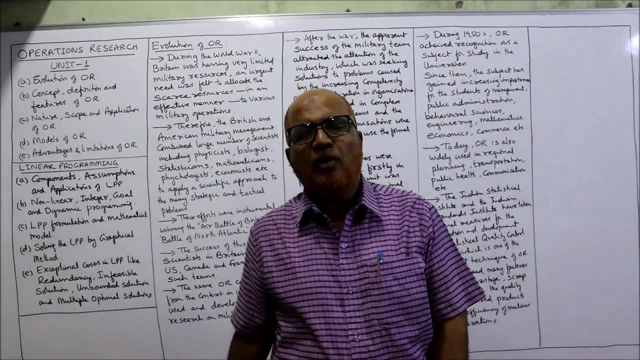 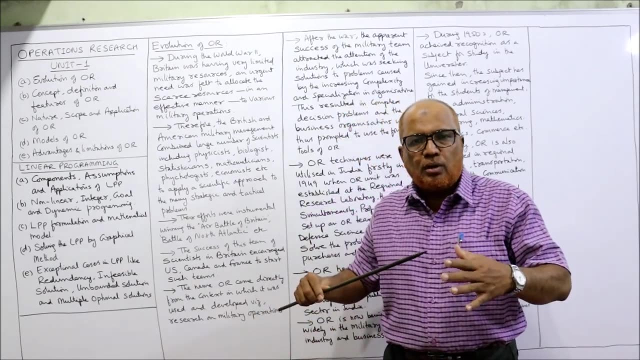 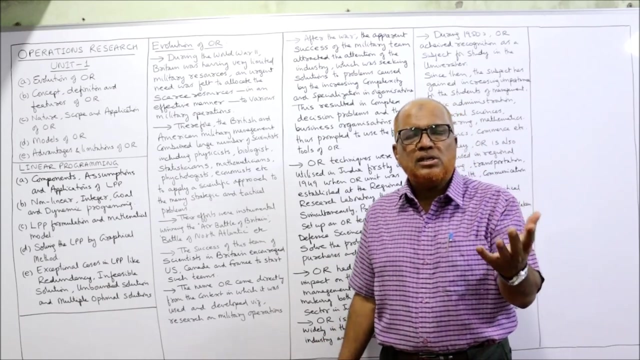 now, evolution of the subject: operation research. actually, operational research means research of operations, the how to effectively utilize the resources. scarce resources, we have scarce resources. by using those scarce resources we have to accomplish some objective. so how to attain the objectives? so, computers, computers alrededor welcoming questions. so number one you haveと. 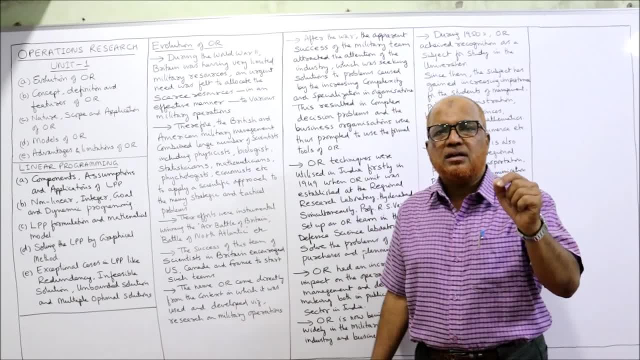 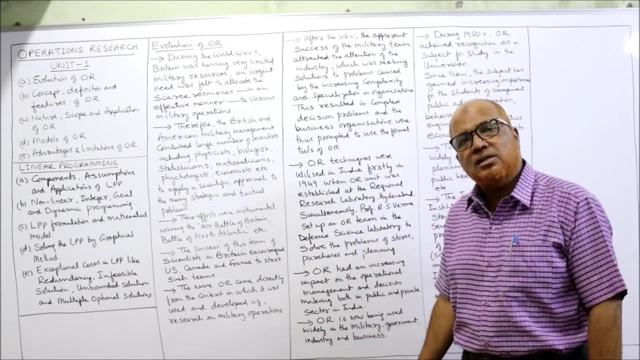 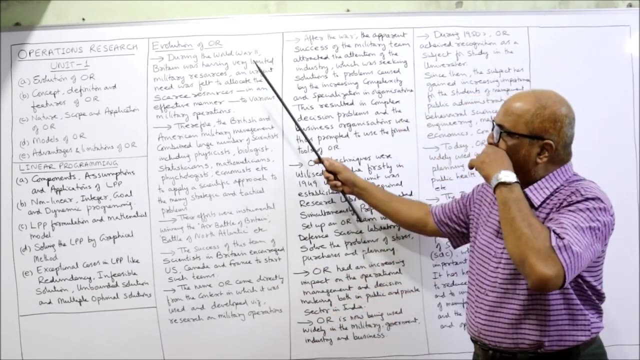 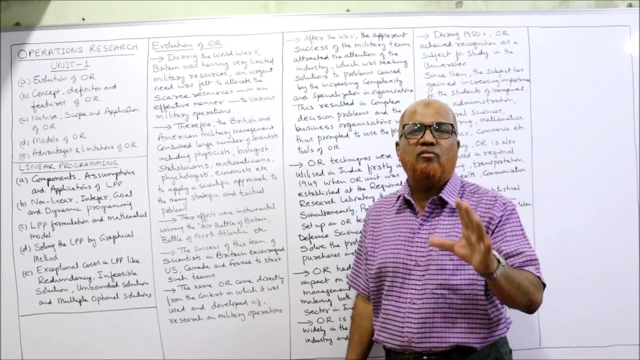 the objective with limited of resources. how effectively we can be able to utilize the resources. that is the main theme of the subject of operation research. number of techniques are there in OR in order to attain the objective. so first of all, evaluation of OR during the world war ii. actually it was originated during world war ii. so during world war ii britain was having 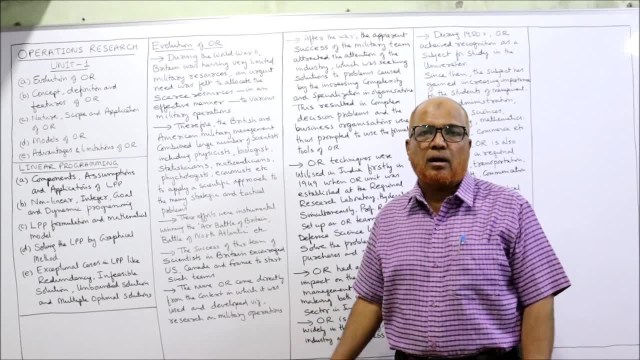 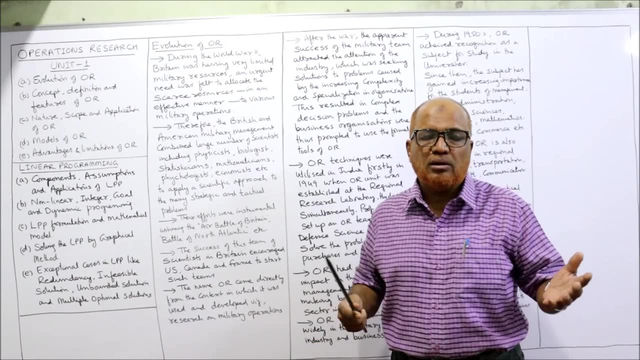 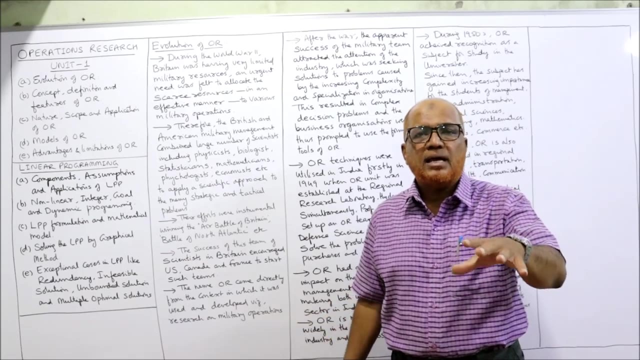 limited resources and they have to win the war. the objective is winning the war, but the resources are very limited. the arms, ammunition and military- these things are limited, but they want to win the war. so how to win the war? by utilizing effectively the limited resources. that is the main problem. 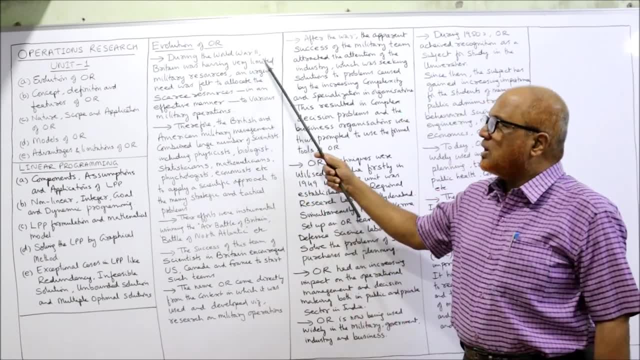 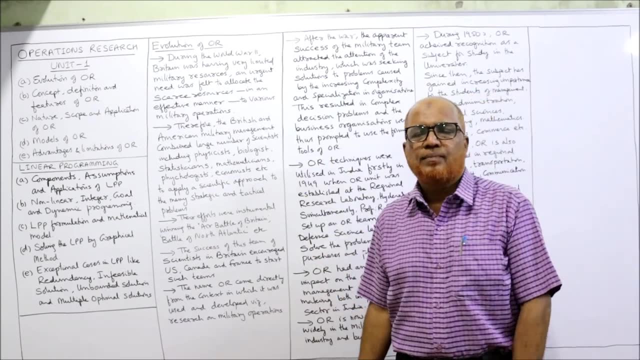 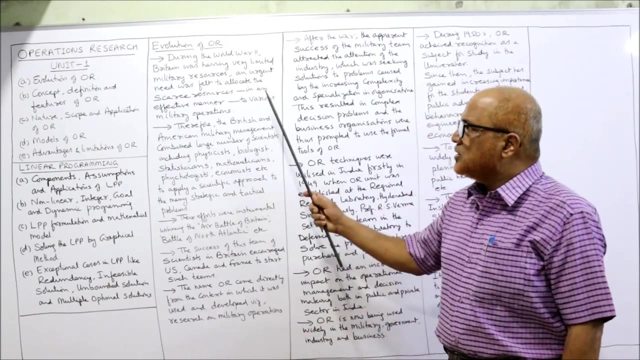 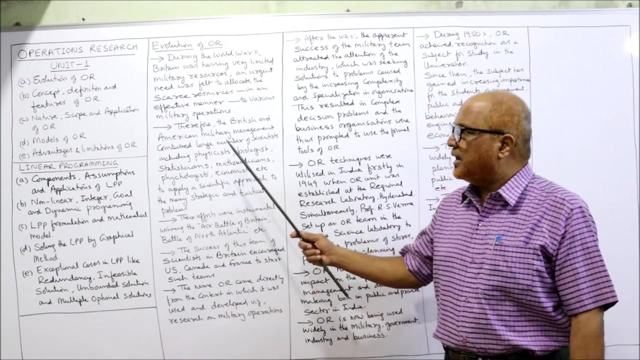 faced by Britain. so Britain was having very limited military resources. urgent need was felt you to allocate the scarce resources, how to utilize the scarce resources in order to achieve the objective of winning the war, so in an effective manner, to various military operations. therefore, the British and American military management combined large number of scientists, including 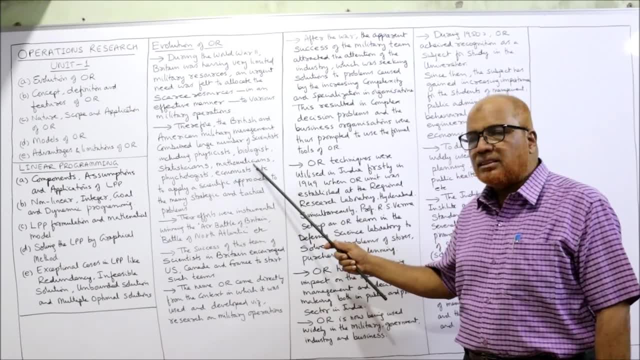 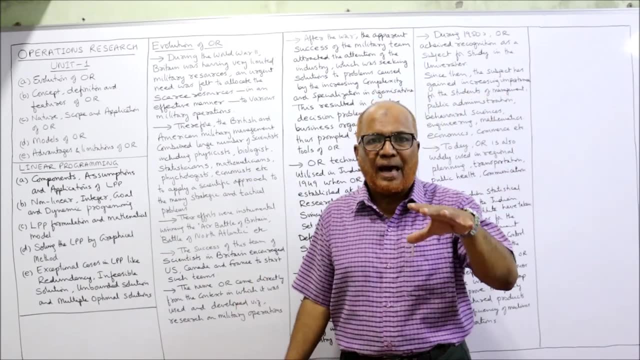 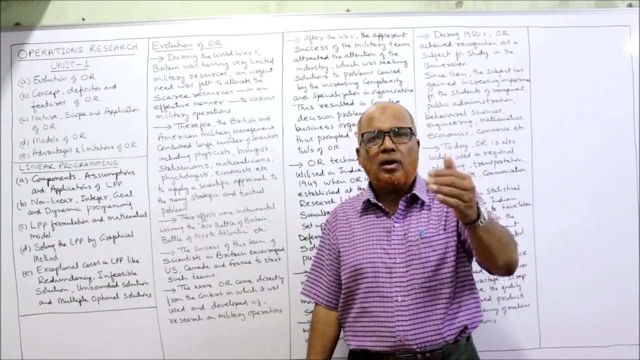 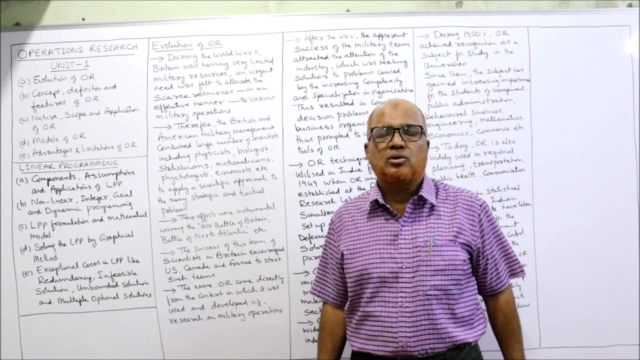 physicists, biologists, statistician, mathematicians, psychologists, economics, etc. so what this British government and American military management team has done? they have called up a number of scientists from different disciplines. they have called up statistician, mathematician, statistician, economist, psychologist, biologist, and they have been given the task to find out a strategic. 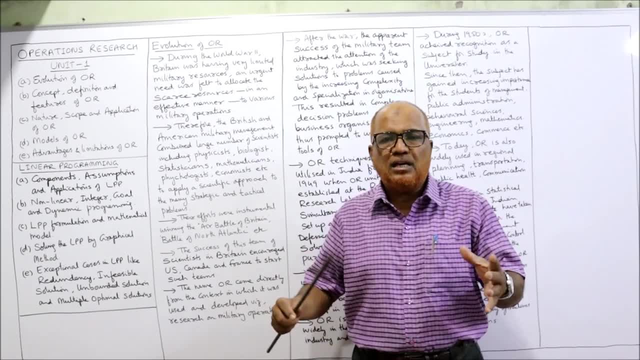 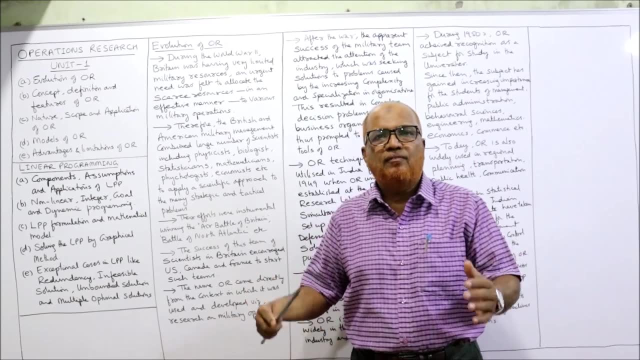 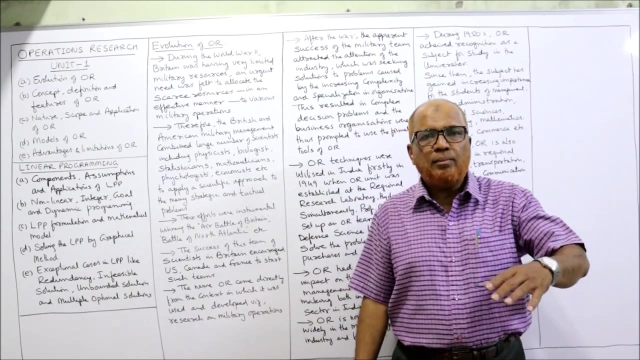 solution of this problem. so every scientist has evolved that we can be able to achieve the objective by this method, by this way, like that. so they have called up different scientists and to apply a scientific approach to many strategic and tactical problems. the government has given them the task how to accomplish this objective by applying your field. 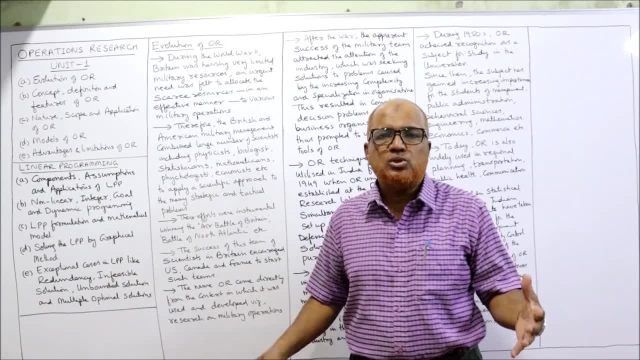 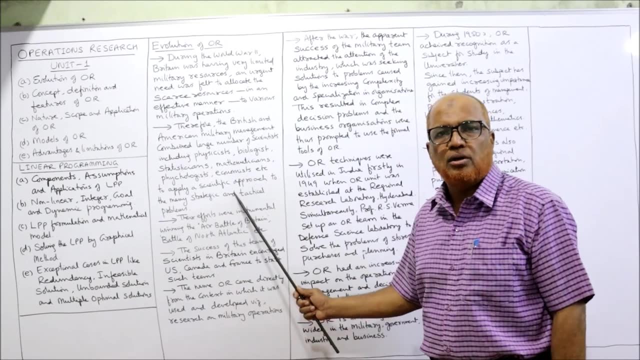 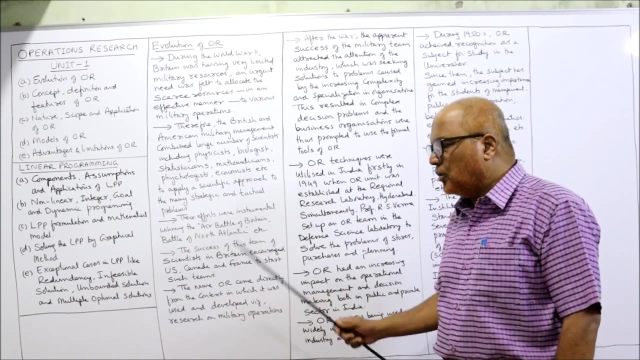 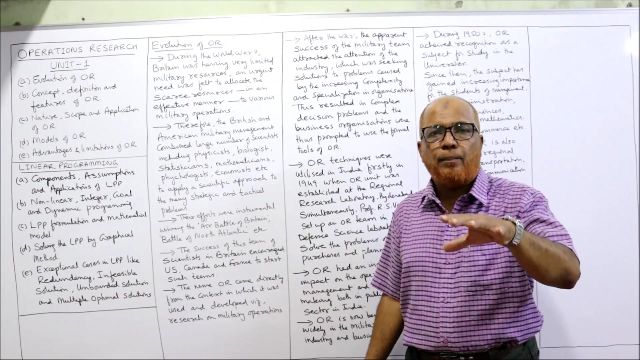 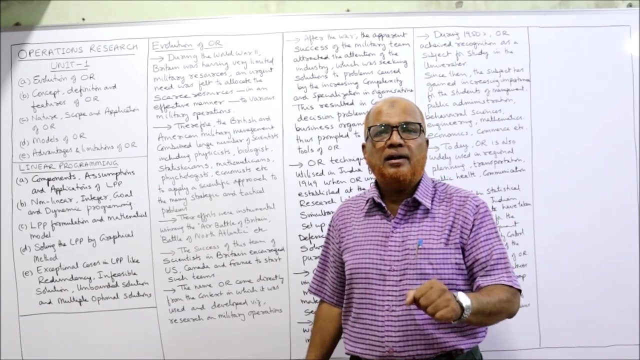 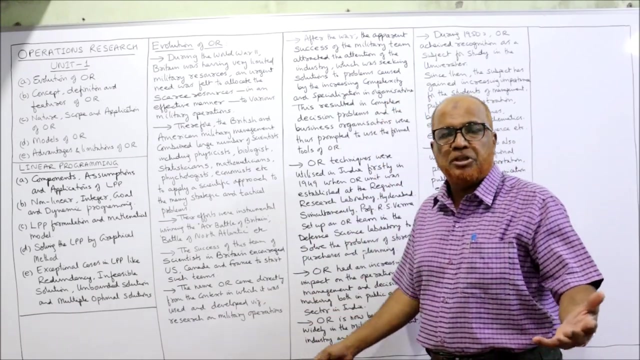 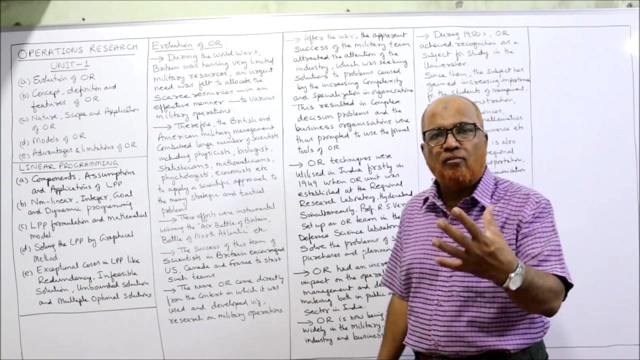 of study, how to find out the an optimum solution to a tactical problem or a strategic problem. that was a main. that was origination of this war: the. their efforts were instrumental, winning the air battle of Britain or Battle of North Atlantic, etc. the outcome of this effort, the outcome of this I mean plan that different scientists are called upon. they have been given the problem to get the solution. ultimately it was instrumental in winning different wars: the war, like Air Battle of Britain, the British has won, and Battle of North Atlantic, mainly the credit goes to the scientists because they have evolved a. 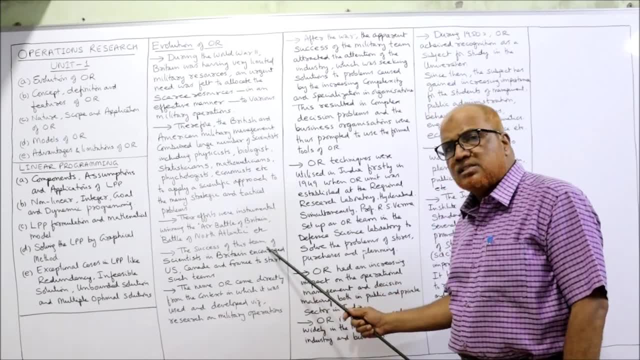 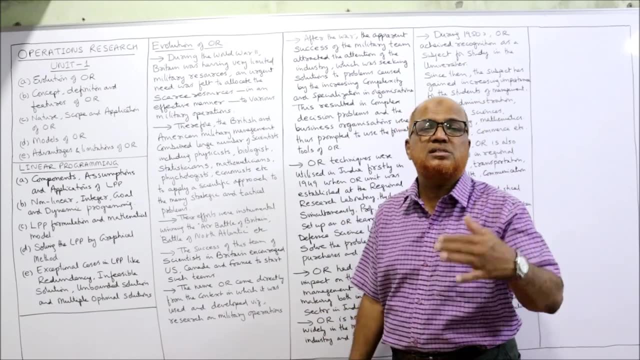 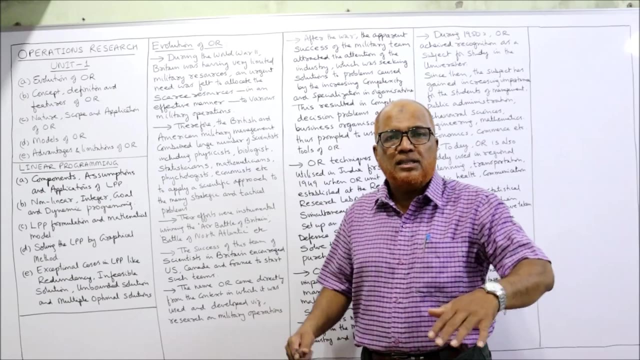 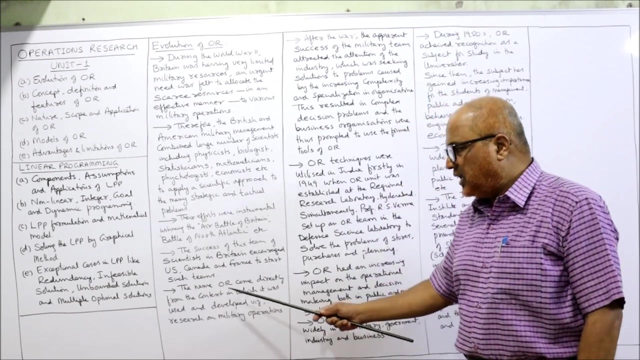 solution for that problem. now, the success of this team of scientists in Britain encourage us- Canada, France- to follow this. I mean technique, to follow this technique. different countries- Canada, France, they have come forward. they have seen that this technique will be effectively utilized in attaining the objective. so the name was came directly from the 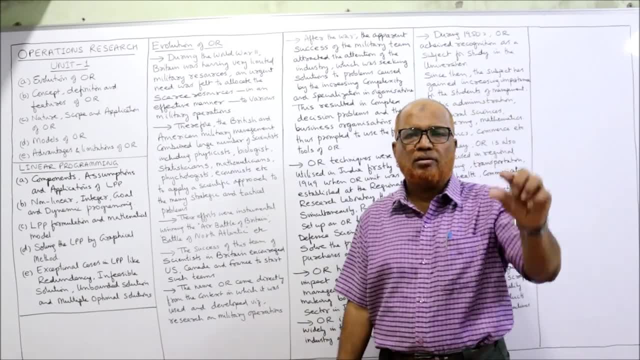 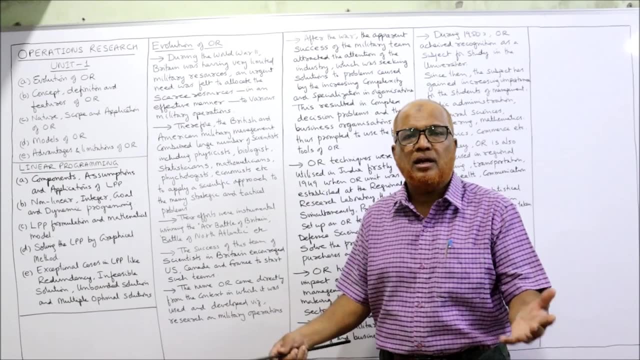 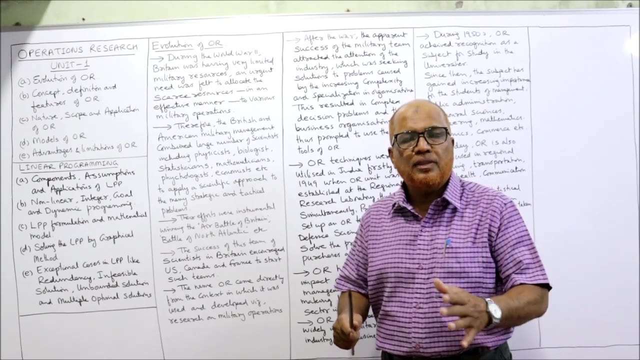 context in which those first years the name Uma came directly from the context in which those first years the name Were perguntども witness to, is basically operation research. this name has come from the first application of this subject where it was applied military, in military operations this subject was applied, so till now the name has 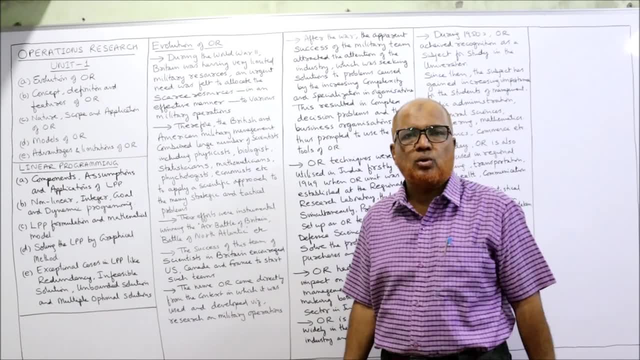 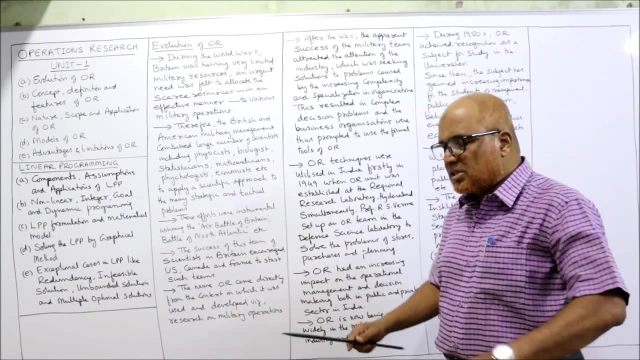 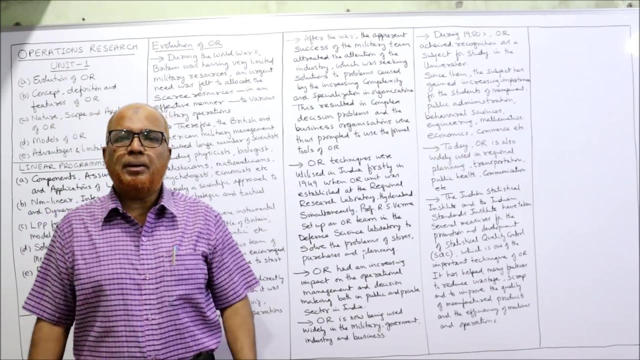 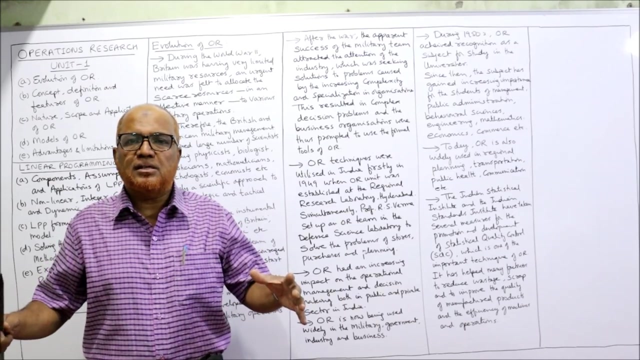 not been changed. the name has been kept as operation research only. so it was started from military operations. now, after the one, that means after the winning so many wars, the concept of this war has been used by business organizations, by industries, by government, by different departments. they have seen that we can be able to achieve the success, we can be able to achieve the objectives. 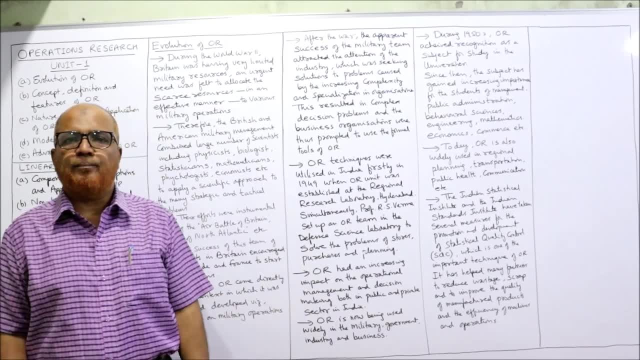 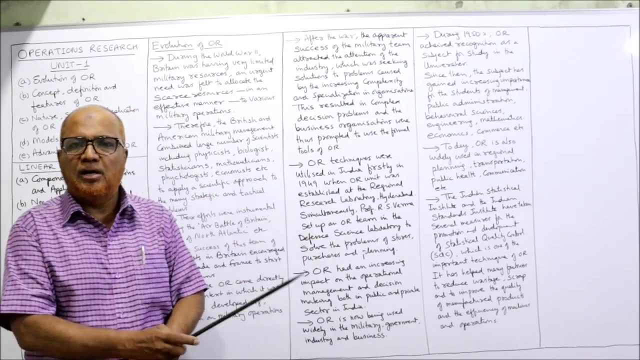 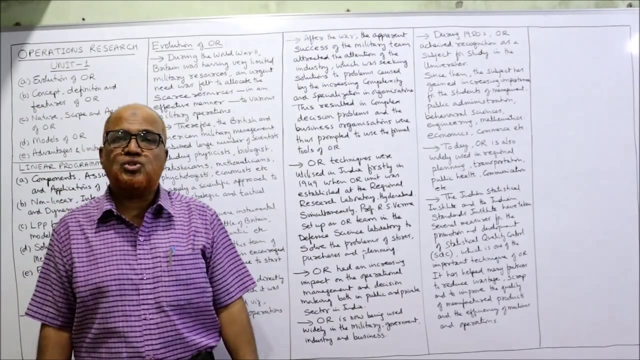 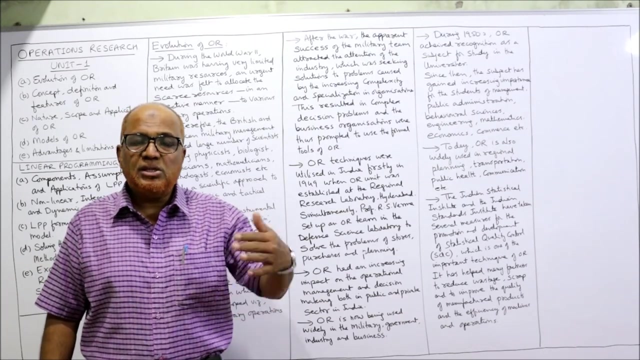 by using this technique of war when we have limited resources and to effectively, effectively utilize those resources in order to attain the objective. so, after the war, the apparent success of military team attracted the attention of industry. the industry people, the business people have seen that this is a better technique. by using this technique, we can be able. 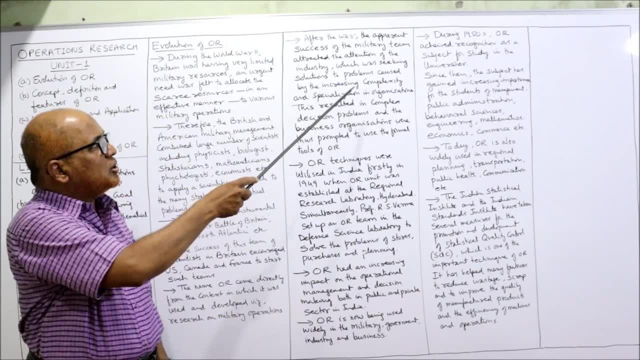 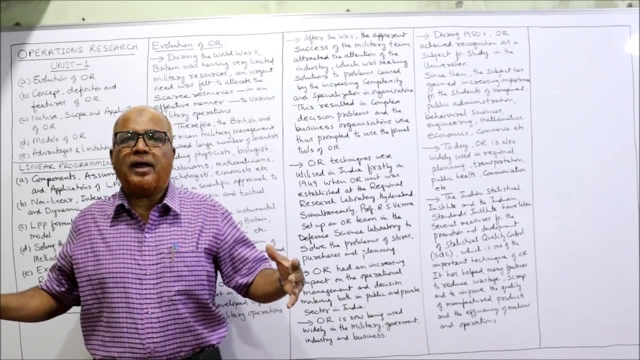 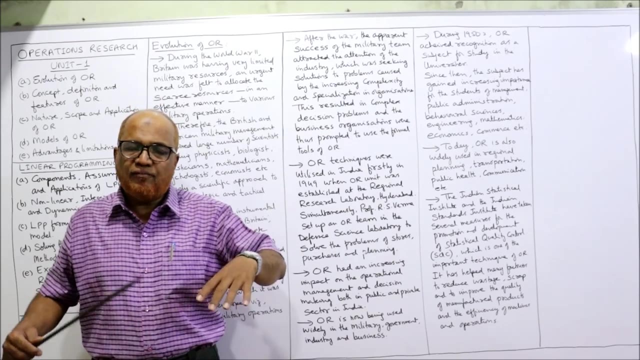 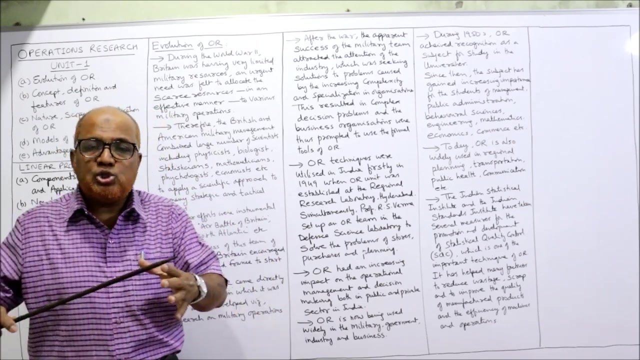 to achieve the different objectives. so which was seeking solution to problem caused by increasing complexity. nowadays, the business, the industries has become so complex due to advancement in technology, due to competitiveness, due to, I mean- different development in different sectors, the business has become, the industry has become more and more complex and due to specialization in the 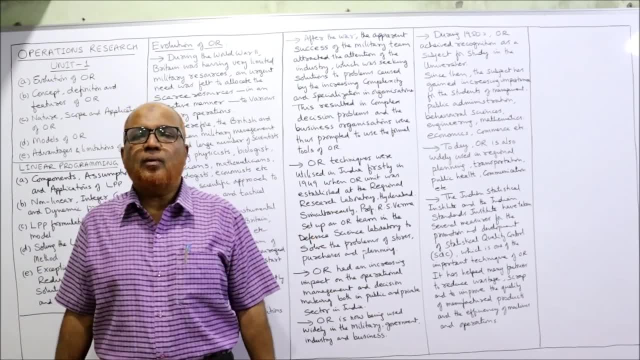 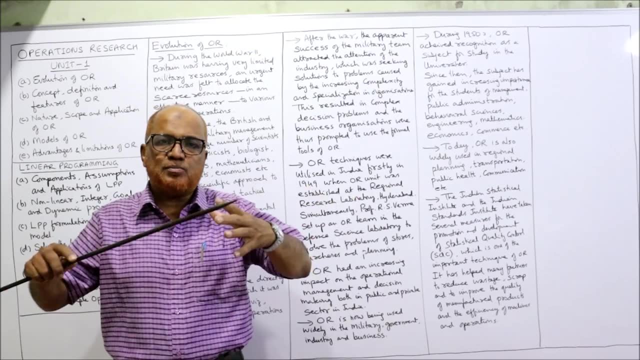 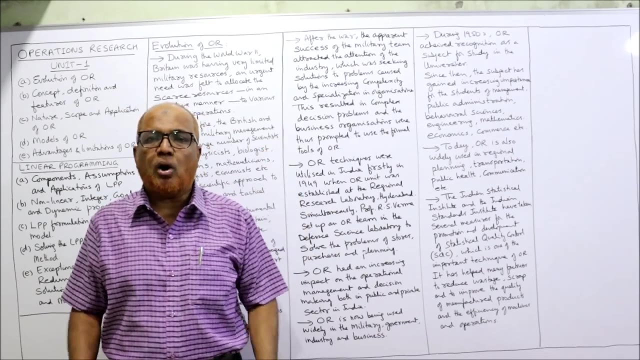 business due to growth of the business. now it's difficult to manage a huge multinational company. the multinational companies are not able to manage the market. they are not able to manage the market having various department ways, branches throughout the world. it will be difficult to manage, control, control such a giant business. so operation research will be very helpful in solving most of the 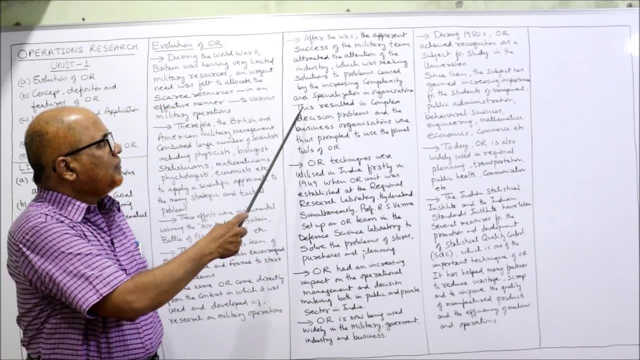 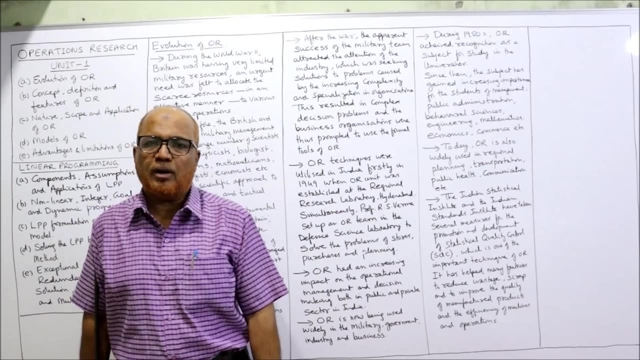 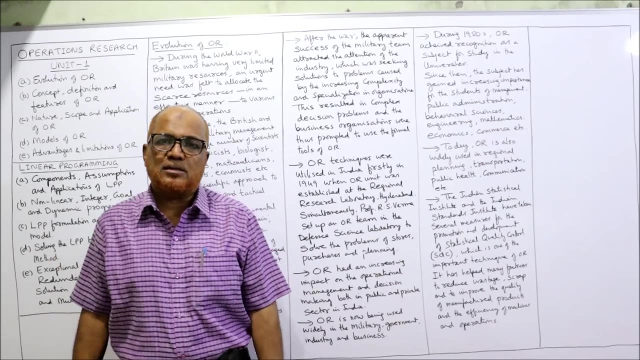 strategic decisions of industries. now this resulted in complex decision problem and the business organization were thus prompted to use formal tools of war. now, as the business grows, industries grows, the problems fade away and the problem is solved will become more and more complex. so in such a situation, to solve the complex problem, the 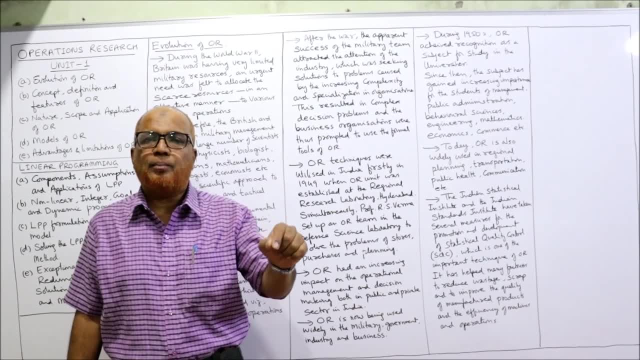 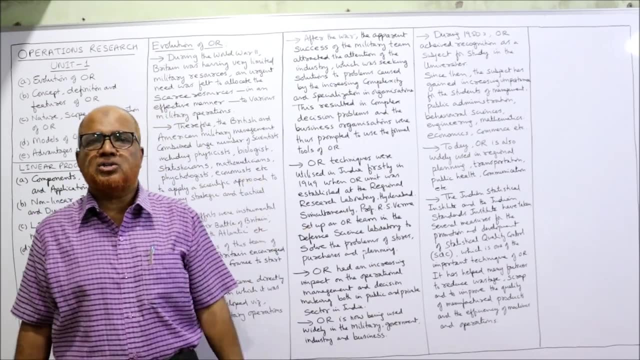 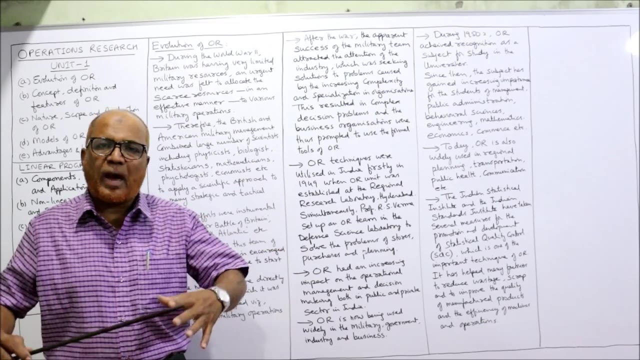 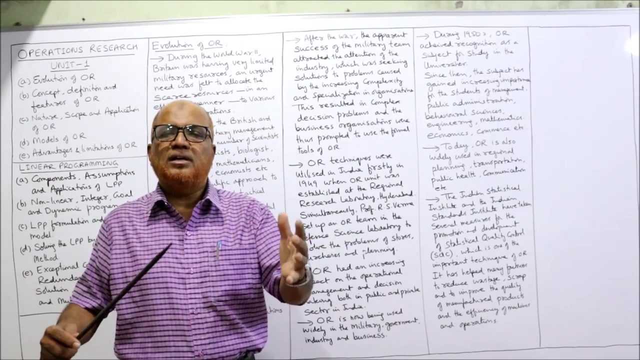 industries are using the techniques of operation research. that means operation research is not confined only to military organizations or military departments. the techniques of or can be equally utilized- very well utilized- by different departments, wherever we have scarce resources and how to effectively utilize those scarce resources in order to achieve the objectives. 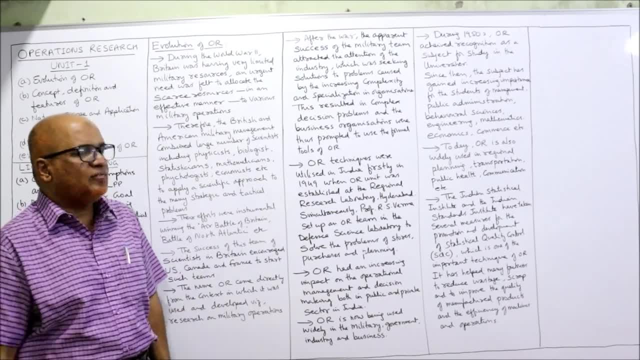 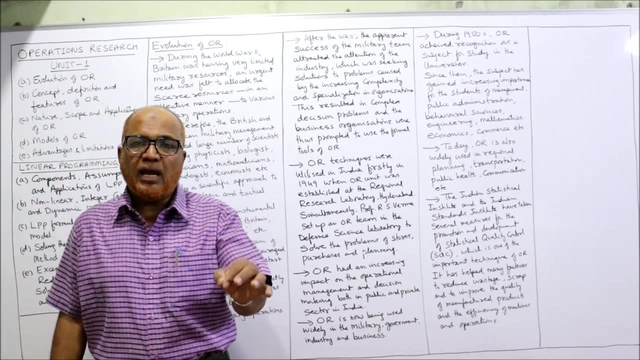 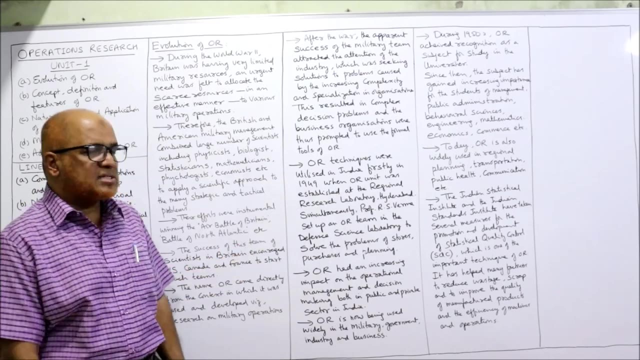 now what techniques were utilized in India. firstly in 1949. now we are studying about the evolution, so it was evolved during Second World War, but in India it was first utilized. this war was first utilized in 1949, when war unit was established at regional research laboratory Hyderabad in Hyderabad. 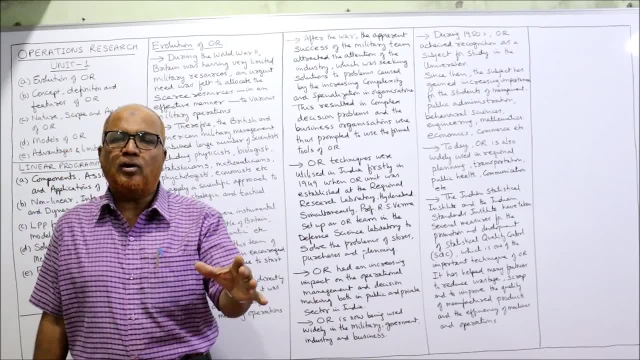 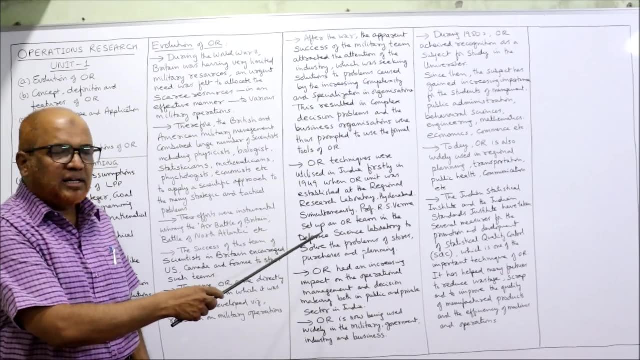 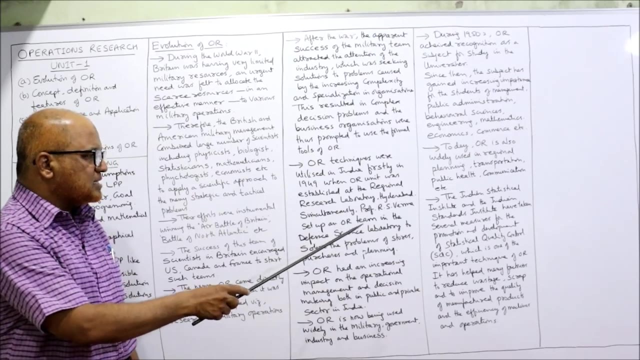 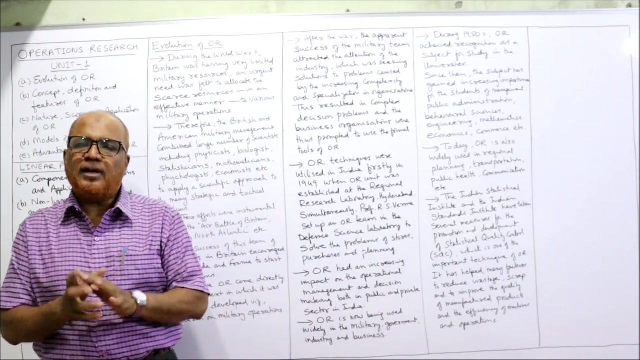 RRL, regional research laboratory. in this laboratory OR technique was first utilized in 1949. later, simultaneously, Professor rs Verma set up a team, set up a team war team in defense science laboratory to solve the problems of stores, purchases and planning. see here OR technique is not confined. 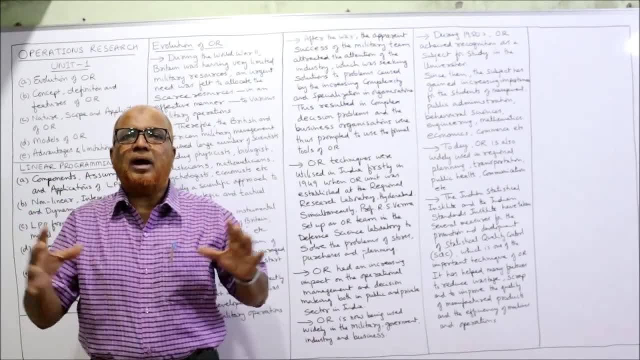 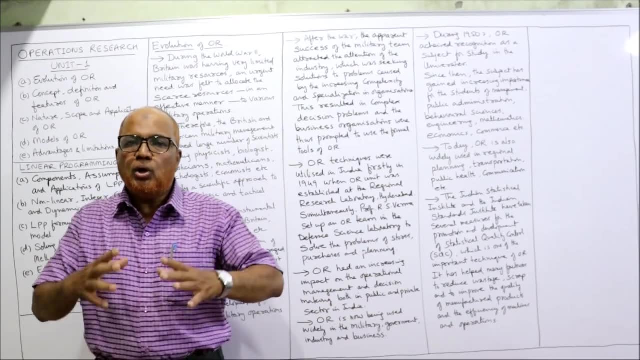 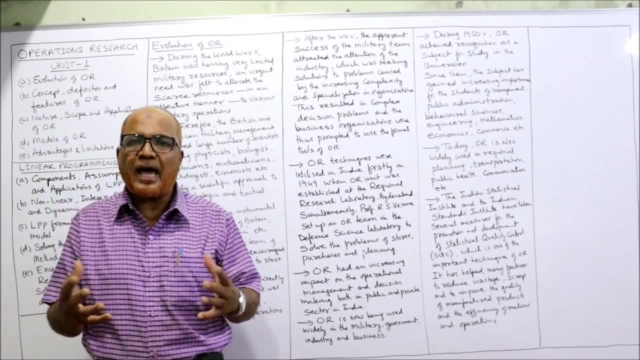 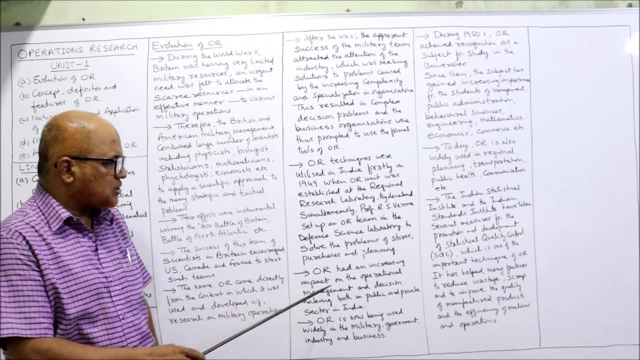 only to military. it can be applied to different departments. so here, Sir RS Verma, he has applied this in different science laboratory to solve the problems of stores and then purchases and planning. For all these things, OR techniques are fully utilized Now, OR had an increasing impact on the operational management and decision making both in public and private sector. 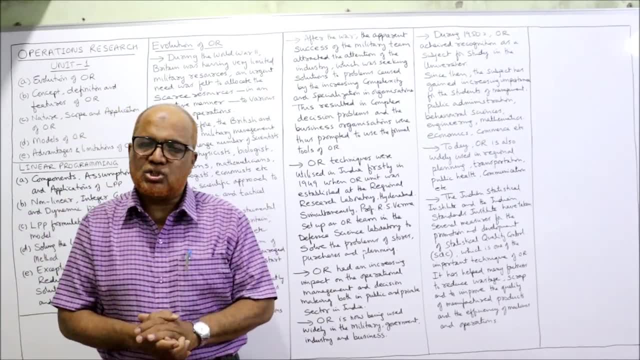 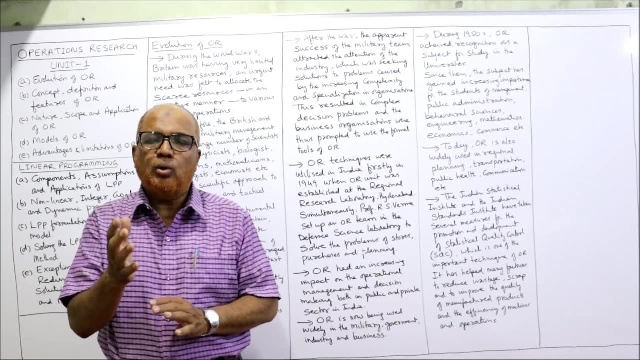 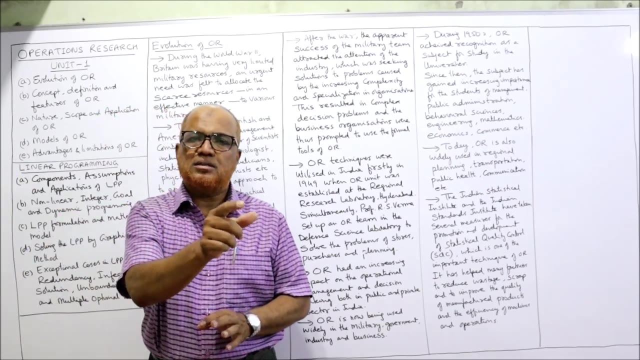 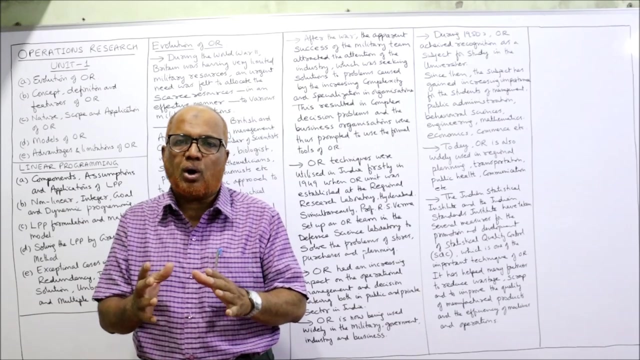 Slowly. the operational research techniques are widely used by management in order to take the decisions. So simply we can say: operational research is a decision making technique. Operational research techniques will be utilized by management in order to solve a complex problem That is OR. 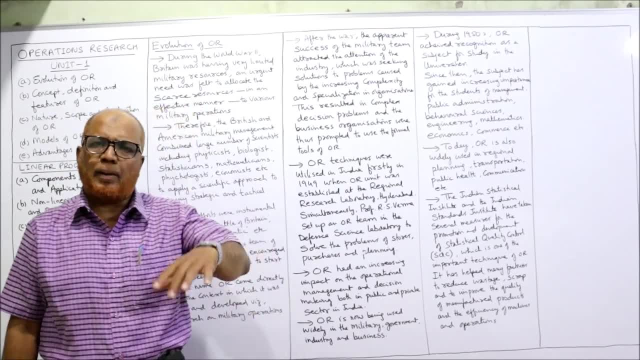 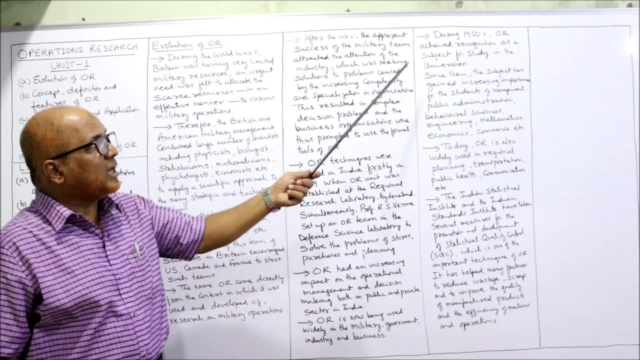 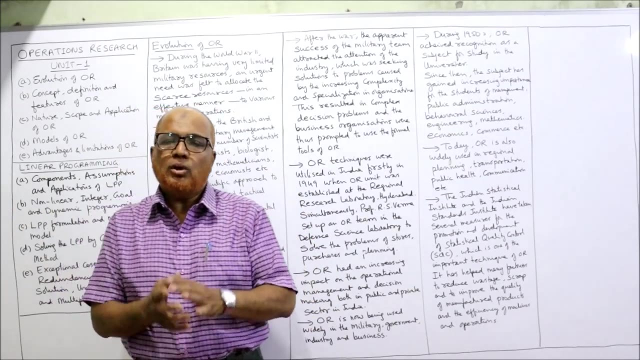 Now it is widely used in any sector, whether it is a public sector or a private sector. it is equally important Now. during 1950s, OR achieved recognition as a subject of study in various universities throughout the world. So during 1950s, the universities have recognized that OR is a field of study. 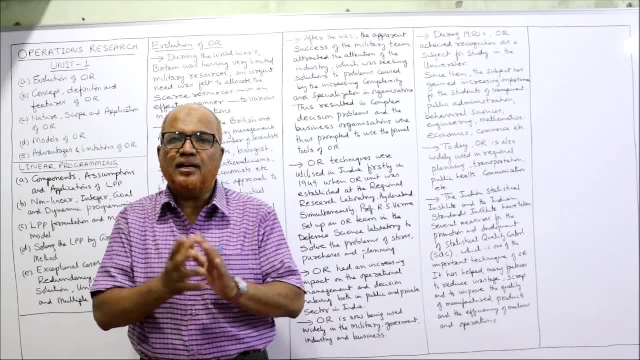 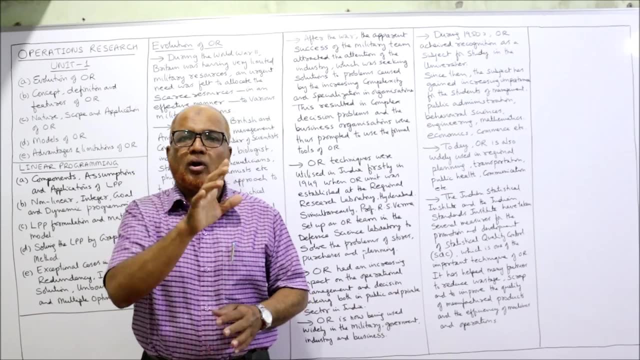 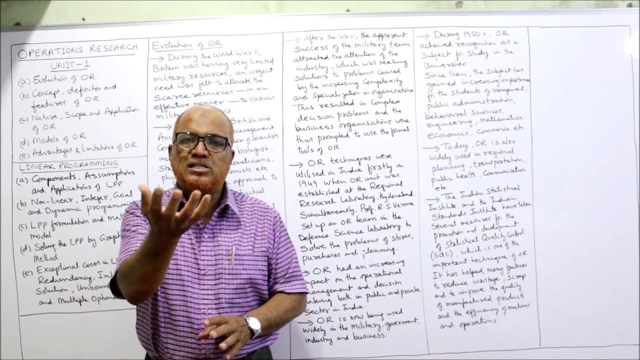 Operational research is a subject of study of different techniques. So university I mean we recognized that this subject should be taught for different graduation, post graduation students, that these are the techniques which can be utilized by management in order to solve the problems. 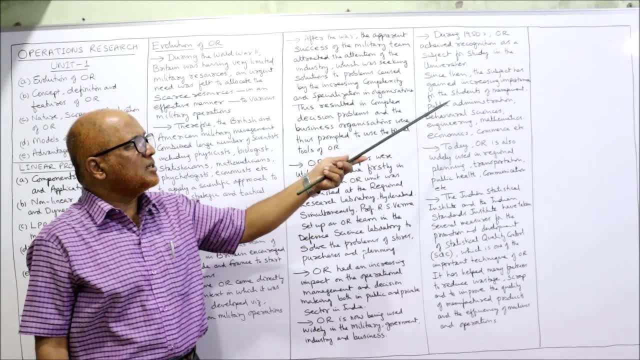 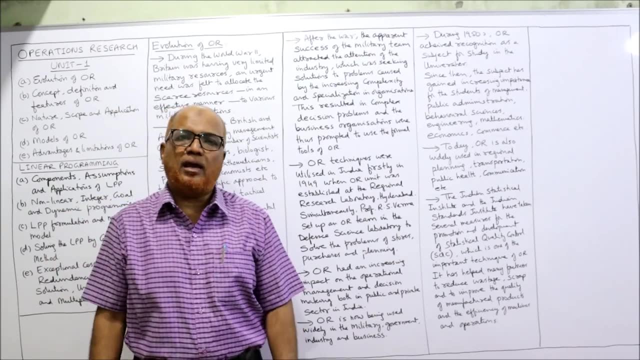 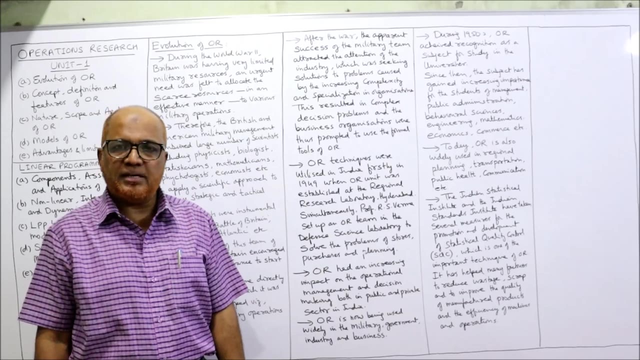 Now, since then, subject has gained increasing importance for the students. That means after becoming a subject in the universities. now this has become very, very important for the students of management, Those who are doing MBA, BBA or BBS, all these students, management students- this subject has become very important. 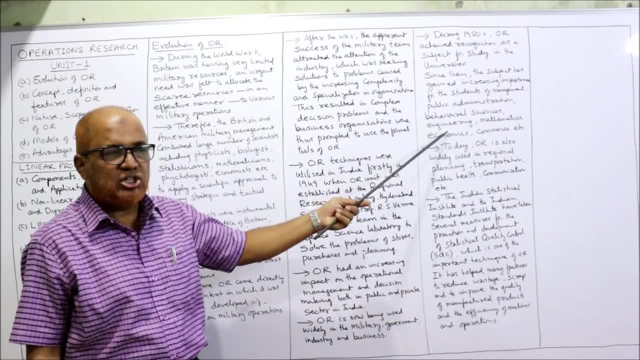 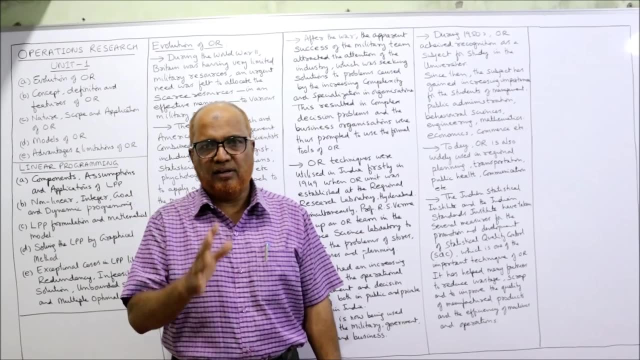 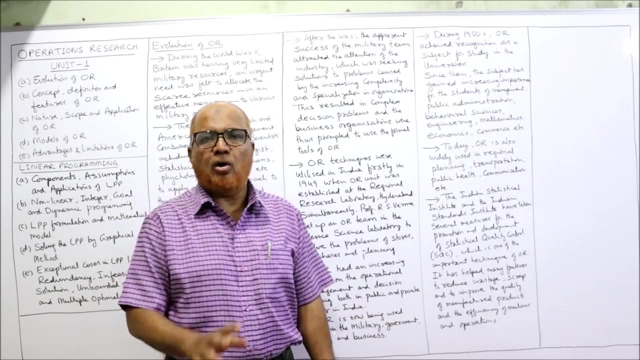 Apart from the public administration, behavioral sciences, engineering, mathematics, economics, commerce- for all these students this subject is very, very important. All the universities' boards have included this subject of engineering, engineering or commerce or economics or management, like that. 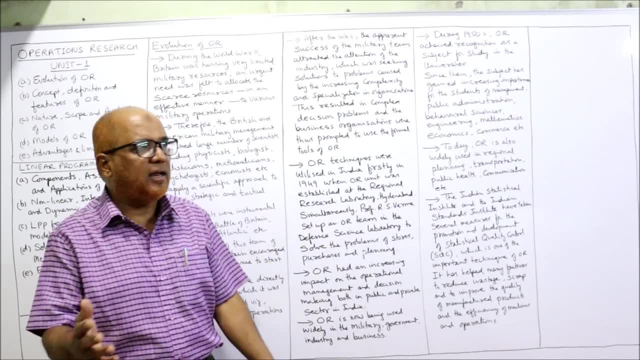 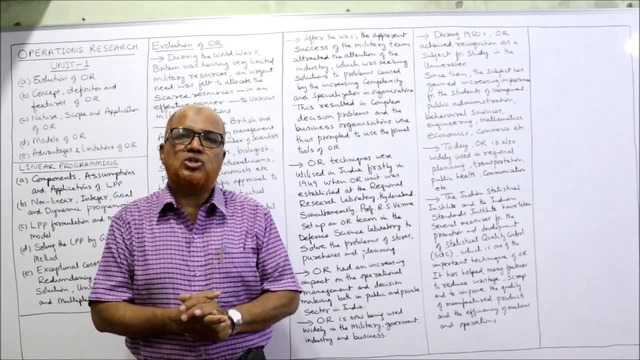 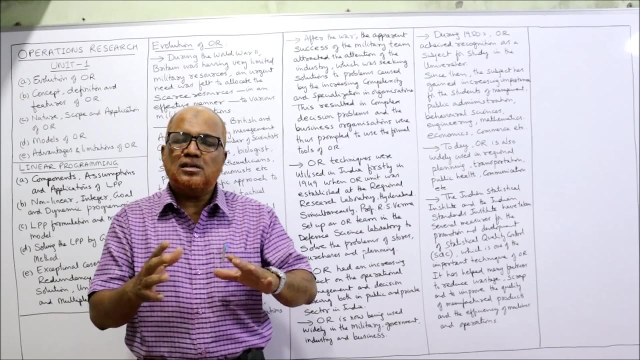 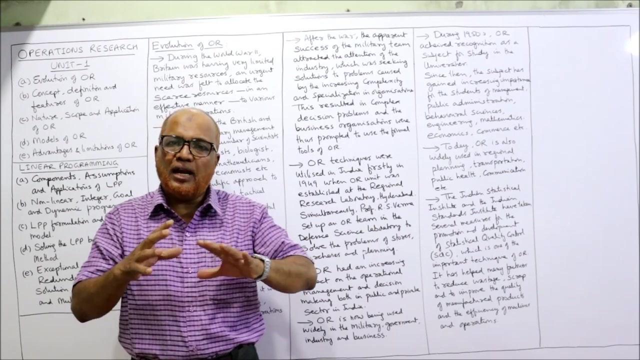 Today OR is also widely used in regional planning, transportation, public health, communication. That means area has widened. The scope of application of this OR has widened. It is not confined only to military or only to business. It is equally applied for communication, for healthcare, for transportation, for assignment, for networking. 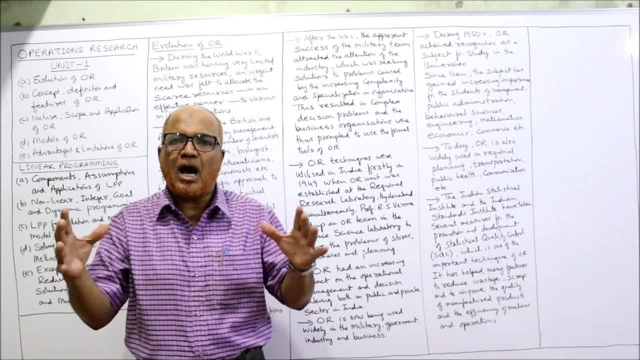 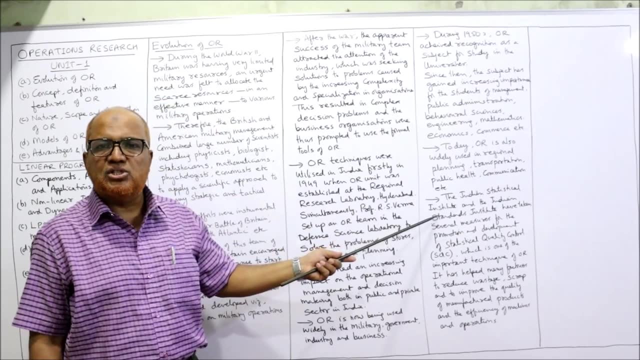 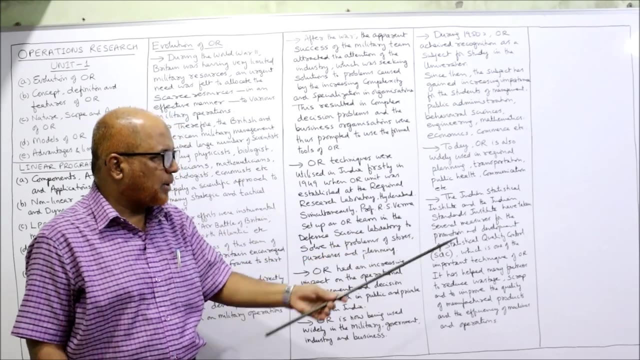 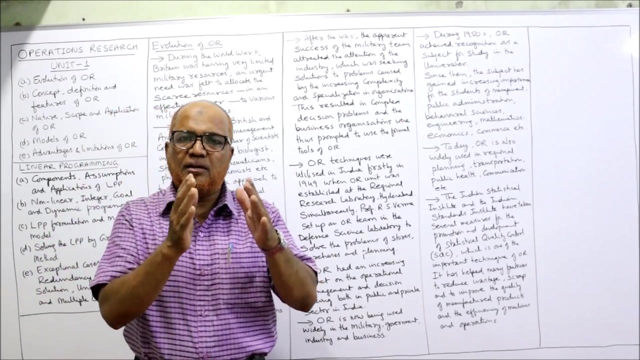 So for different purposes, different areas This operational research is being utilized. Example I have given here: the Indian Statistical Institute and Indian Standards Institute, ISI, which we call, have taken several measures for the promotion and development of Statistical Quality Control, SQC, and which is an important technique of this operational research. 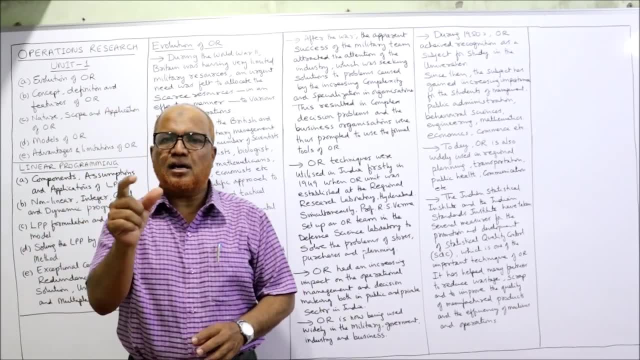 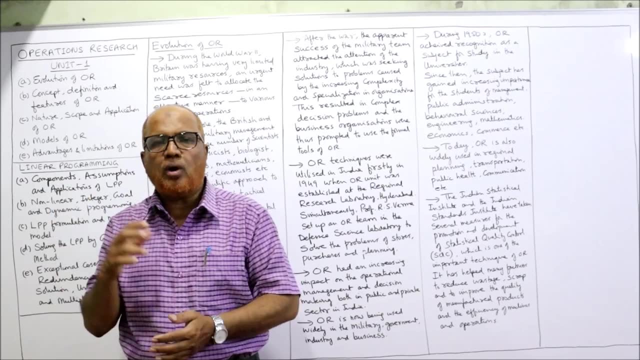 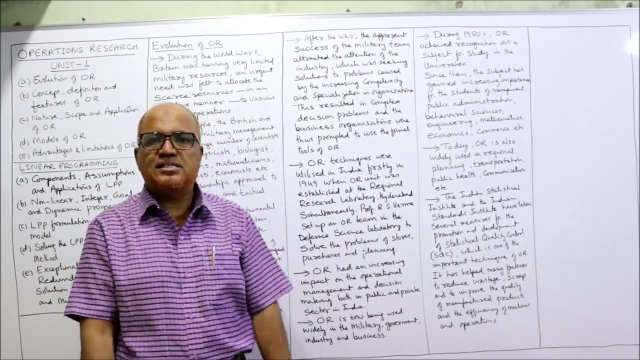 In operational research. one of the technique is Statistical Quality Control- How to control the quality statistics Statistically? the technique has been suggested by OR and this SQC has become very important tool for Indian Statistical Institute and Indian Standards Institute. They are using it to control the quality, which is one of the important things. 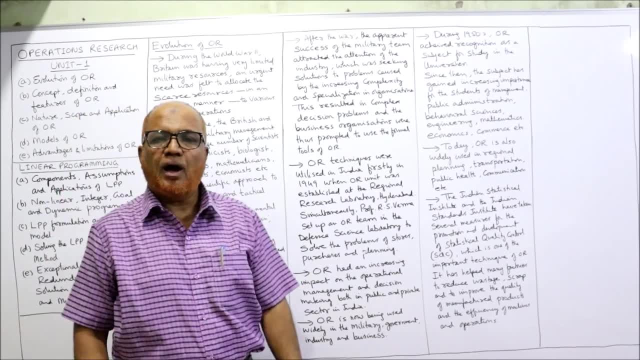 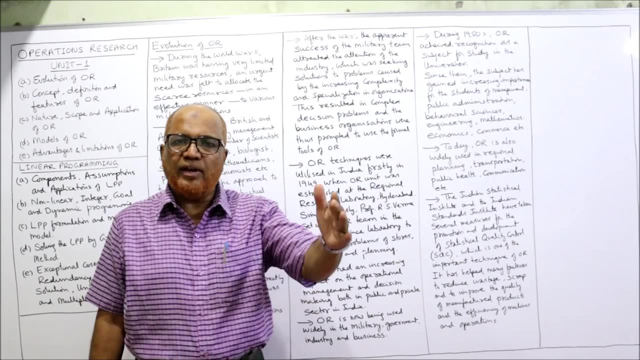 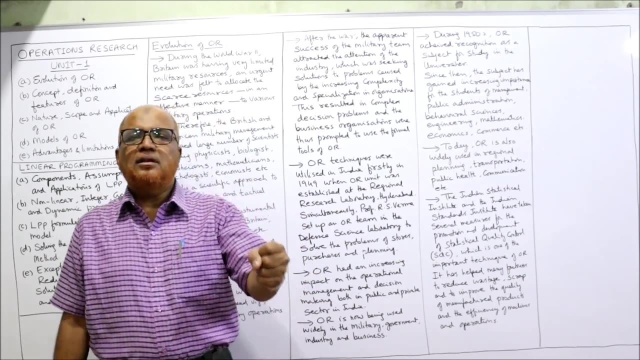 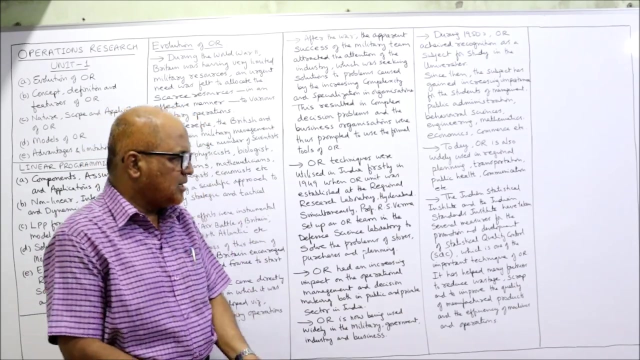 It has helped many factories to reduce wastage. How this OR will be helpful. It will be helpful in removing the wastages, in removing the inefficiencies, In removing the idle time. that means the resources can be effectively utilized if we apply OR in the factories. 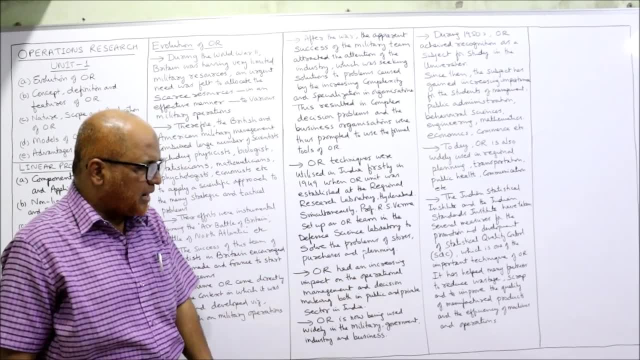 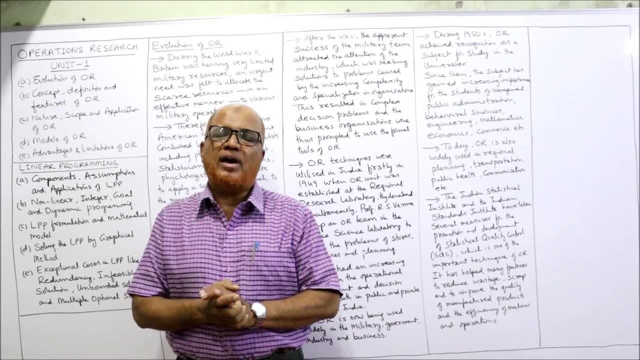 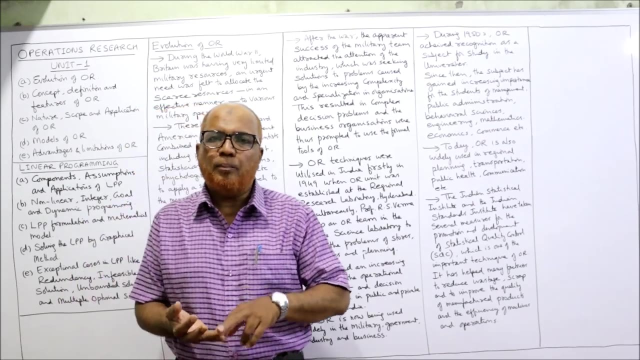 So reduce wastage, scrap and improve the quality of the manufacture products and the efficiency of machines and operations. Ultimately, this OR will be very, very helpful in increasing efficiency of men, machines, material operations. All these things will be facilitated by using this OR technique. 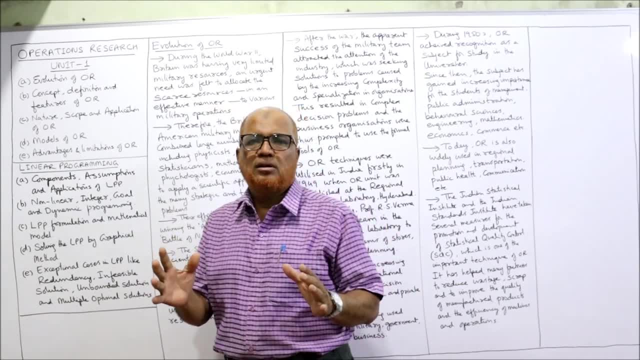 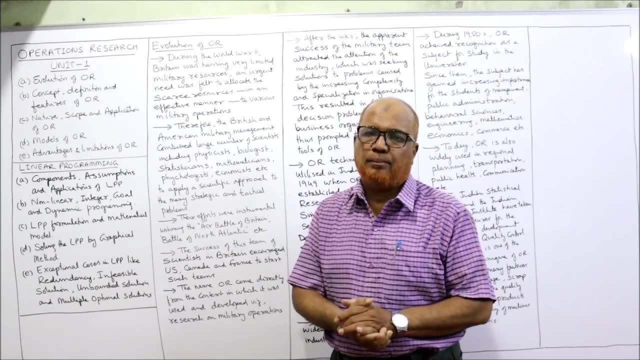 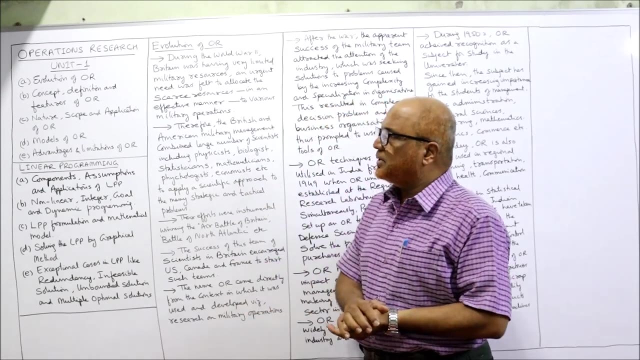 So in this video I have explained you just the evolution stage, when it was evolved, how it was developed over a period of time. Next video, Insha Allah, I will explain the nature concept. First I will explain the concept definition and features of operational research. 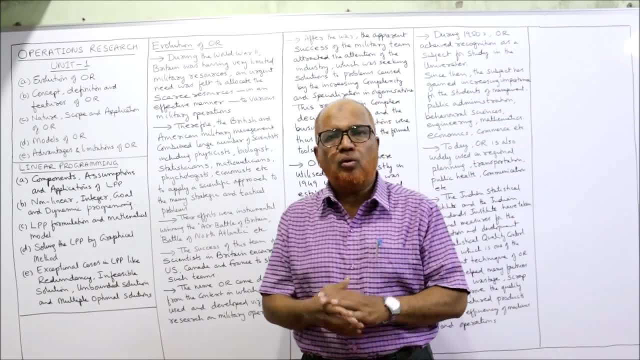 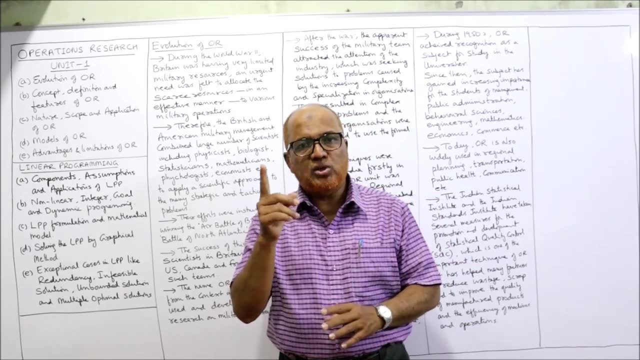 And secondly, nature, scope application, Then OR models, Then SQC, Then advantages and limitations. So if you want the perfect knowledge, watch all the videos from beginning till end, Don't skip in between And remember. one more point I want to tell to my dear students: 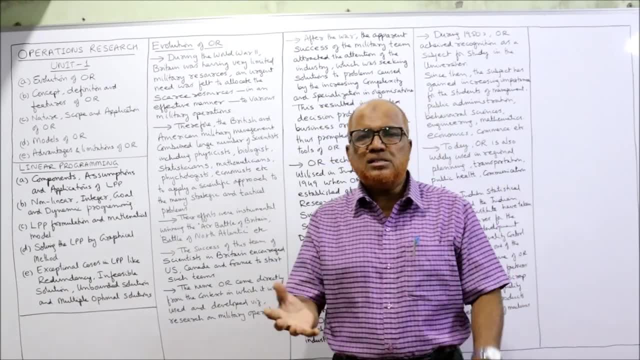 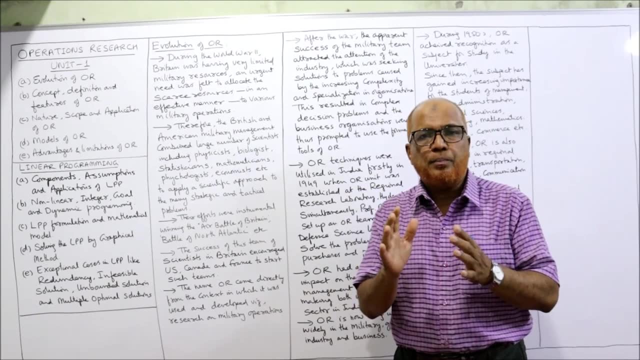 Don't focus only on problems. The theory is the foundation stone. The problems are based on the theory. Don't ignore the theory. Have some patience. I mean, write some notes while watching the videos. Make some notes, Make some points. 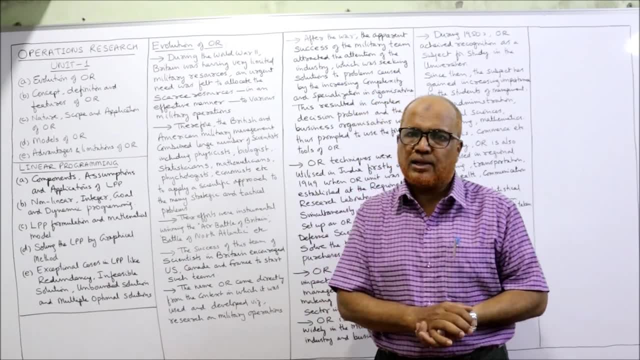 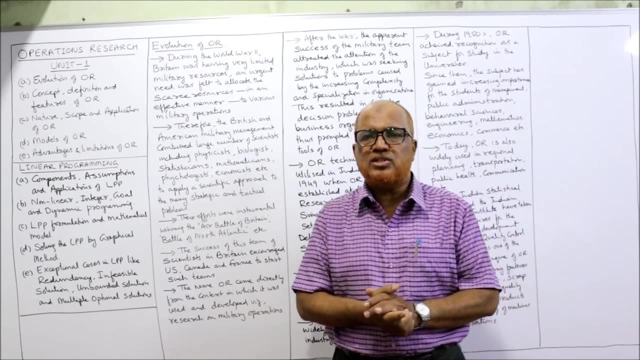 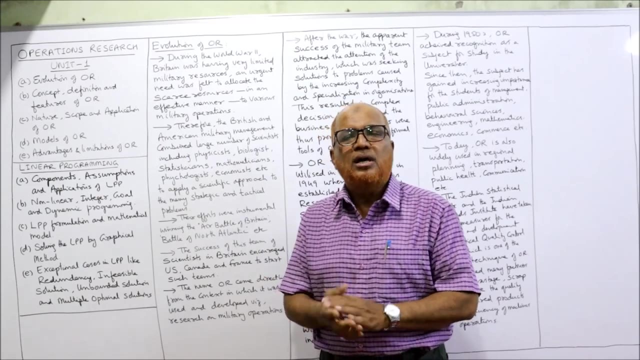 Then only you can get maximum benefit from my lectures. So, Insha Allah, we will continue the next topic in the next video. So if you are new to my channel, give a like, Share my channel among your friends, among your groups, so that more students can watch the video and enhance the knowledge. 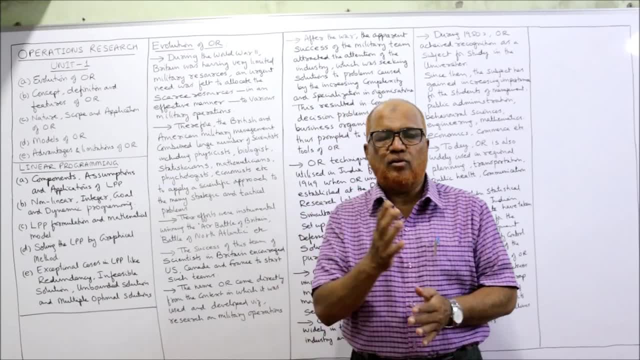 Give your comments on my videos. Subscribe my channel, if you have not yet subscribed, And buy the super thanks which is given below my video. Insha Allah, we will continue in the next video.